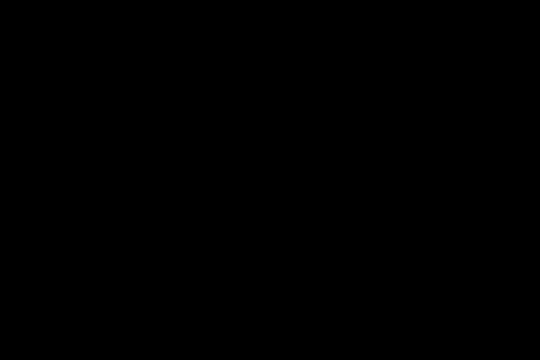 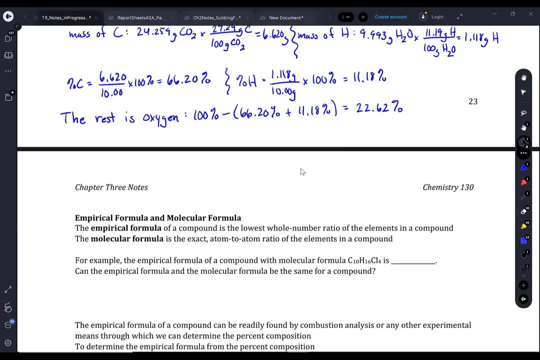 Good, All right everyone. So we're going to continue on. The last thing we've done is we've done a simple combustion analysis question, And what we're going to find is I'm going to start taking all of these questions here and combining them into kind of one large question, And then, after doing that, 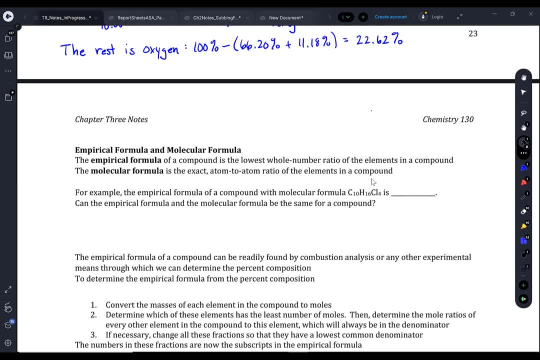 we'll go through another question that's similar, that combines all three parts. So we looked at combustion analysis. And why is combustion analysis useful? It gives you the The what Percent composition. Good, Good, At least for some elements it does. 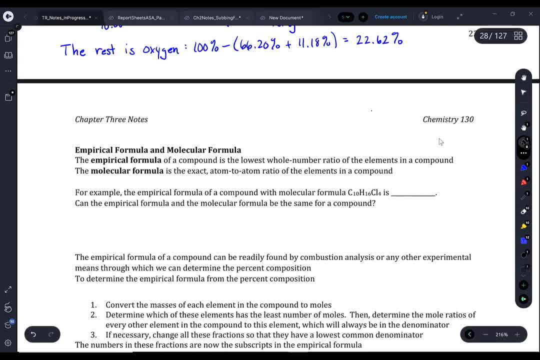 Carbon hydrogen and oxygen. Now what we can do with that information is we can determine the empirical formula, And if we have even more information we can find molecular formula. The empirical formula- kind of meaning formula by experiment- is simply going to be the lowest whole number. ratio of elements to elements. 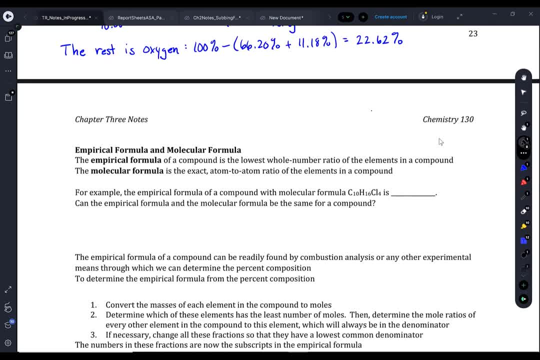 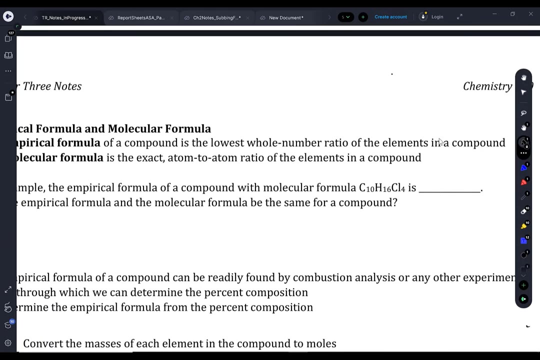 So what we do is, if we know the formula, it's going to be in the lowest possible ratio. You couldn't get it any lower. So, for example, if you were to look here at this compound that has a formula of C10H16Cl4, what would be its empirical formula? 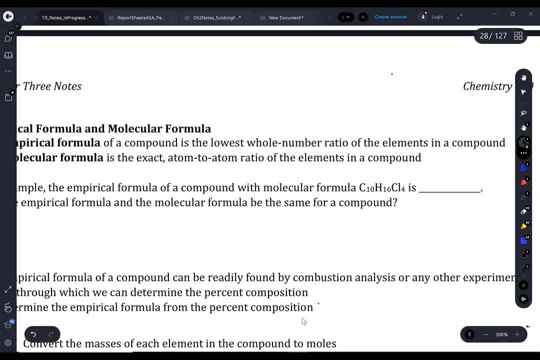 In other words, what number can I divide all of those by? Yeah, two is the largest number that divides into all of those evenly, So I'm going to divide each of those by two. So C10 would be C5.. H16 would be H8. 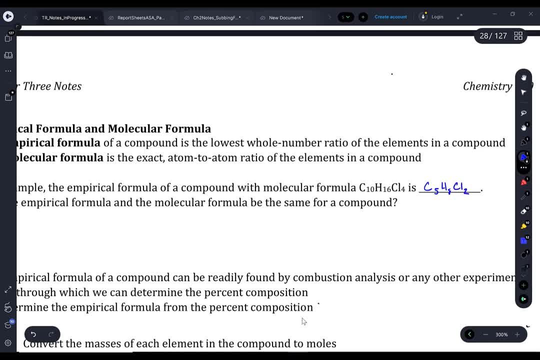 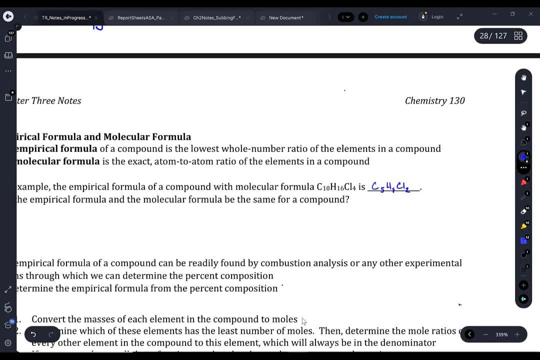 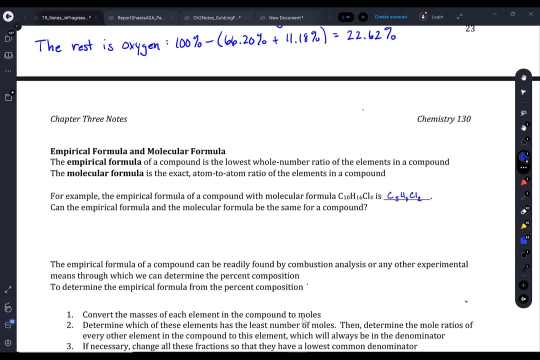 Cl4 would be Cl2.. Right, So we can't divide that any lower. Can the empirical and molecular formula be the same for a compound? Well, let's take a look at a compound. So, for example, here is the Lewis structure. 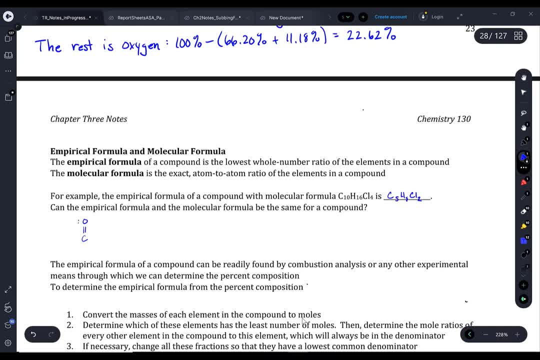 It's a compound of formaldehyde And if I look at that, what is its molecular formula? Starting with carbon, How many carbons are there? One. How many hydrogens? Two And oxygens One, Since as soon as you see that any of the elements has a coefficient of one. 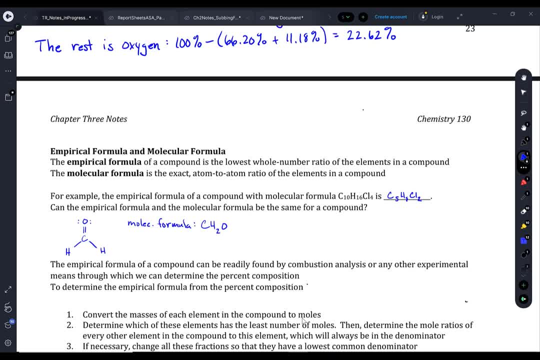 you know you can't get it any smaller, right? You're not going to be able to divide the numbers any smaller. Okay, And so in this case, this is also the empirical formula. Okay, Okay, Okay, Okay Okay. 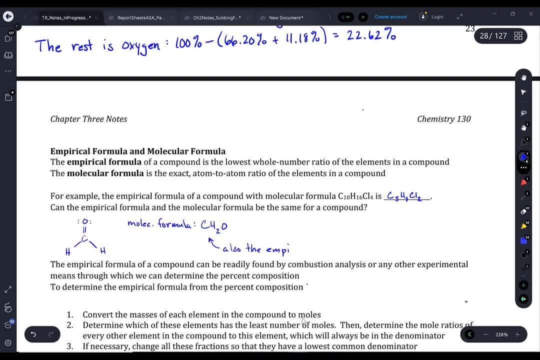 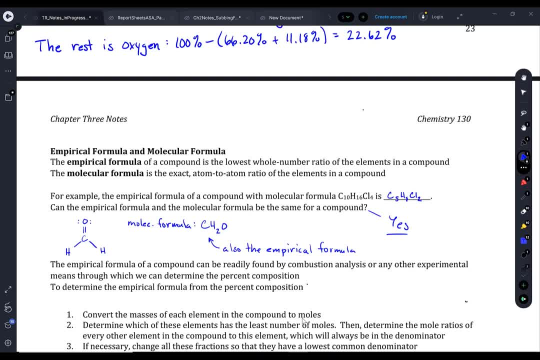 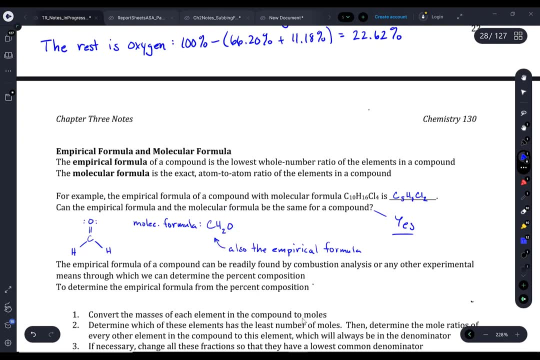 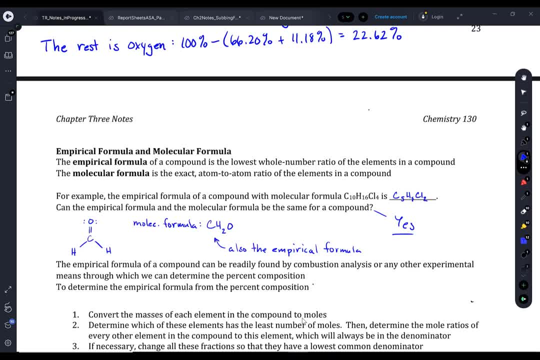 It just has to be. all of these numbers are a multiple of some other number. Oh, you don't have to give me a name, Just give me a formula. Are you sure of anything? Yeah, It doesn't work, No, no, Okay, So I'm saying: different molecular formula, So different. 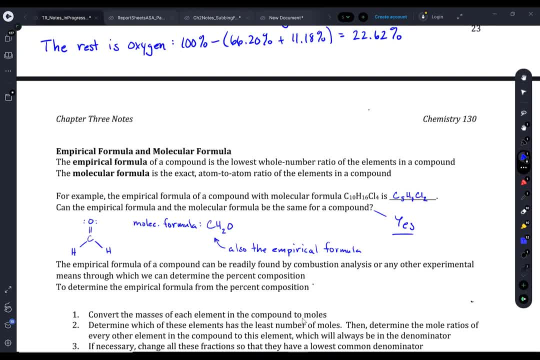 number of atoms. same order, but different formula here. Maybe I'm not being clear. Good, C2H4.. O2.. Good, So in other words, I'm just multiplying all of these by two, or I could multiply by three. 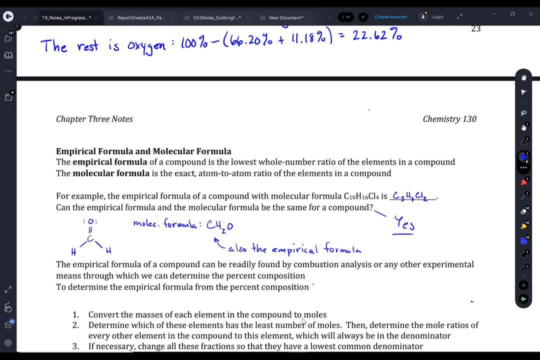 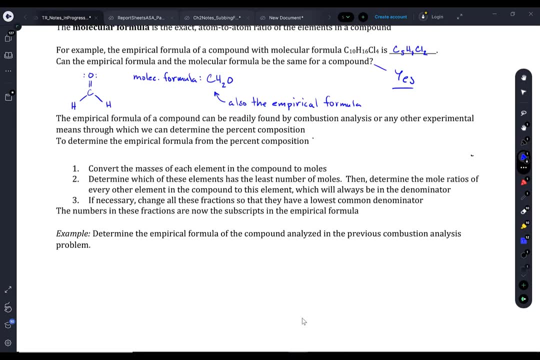 or I could multiply by 20.. C20H40O20.. Those would all have that empirical formula, but a different molecular formula. right Good. Now the way that we find an empirical formula by combustion analysis is the first thing that we need to do is we have to get the masses of any. 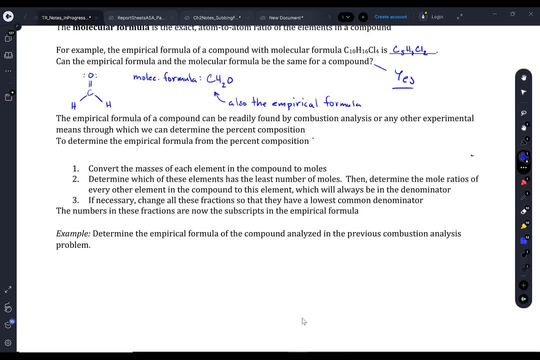 elements that we have and then convert them into moles. Once we have the moles, what we do is we then come up with a smallest whole number ratio between each of the elements, And when we do that, the element with the smallest number of moles 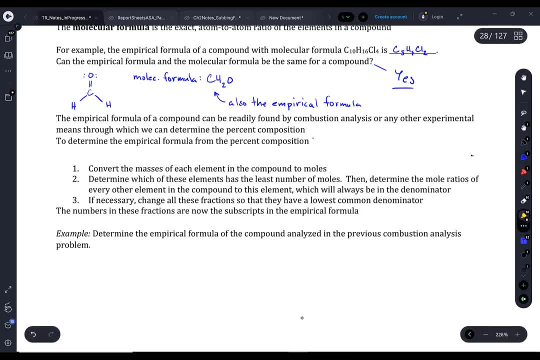 will always be the denominator, as we will see. Otherwise this won't work well. And then, if for some reason the denominators are different, you have to give them the same denominators by finding a lowest common denominator. Now, talking about this is kind of pointless. 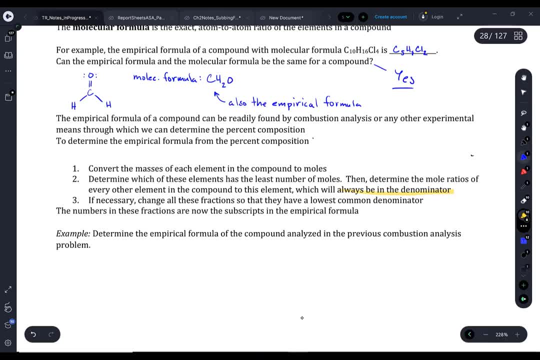 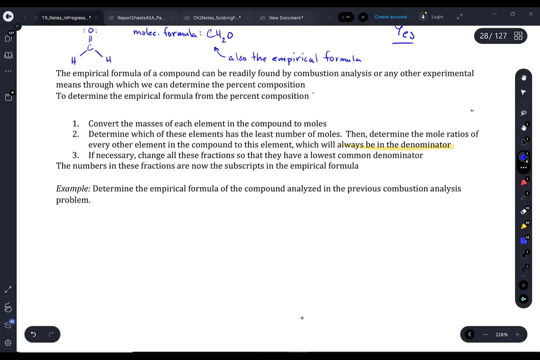 so it makes more sense to just do this as a problem. So I'm going to continue the problem that we just did, which was a combustion analysis, by taking the data that you were given and using that to calculate the empirical formula. So before I begin, I need the percent carbon, percent hydrogen and the percent of oxygen. 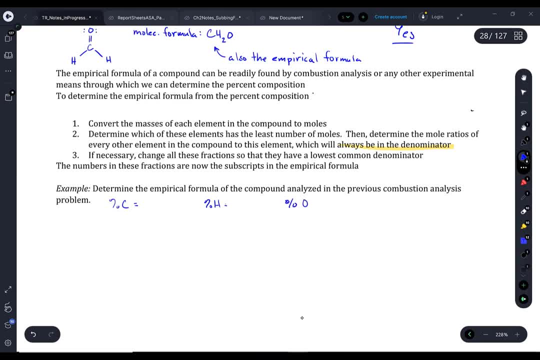 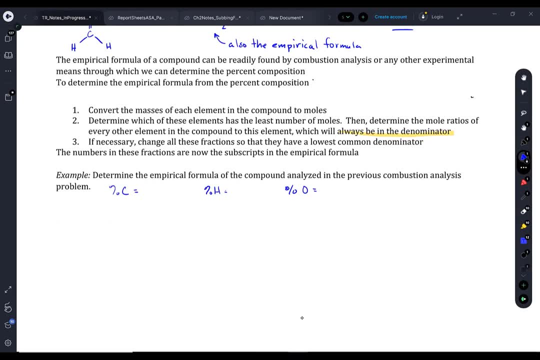 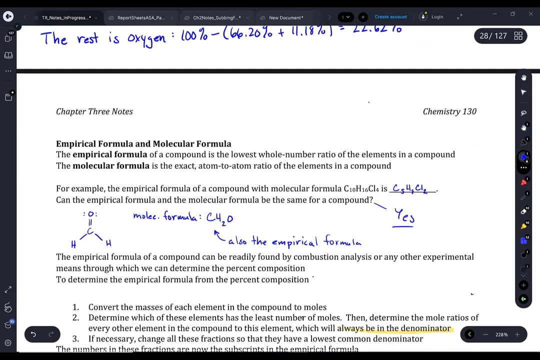 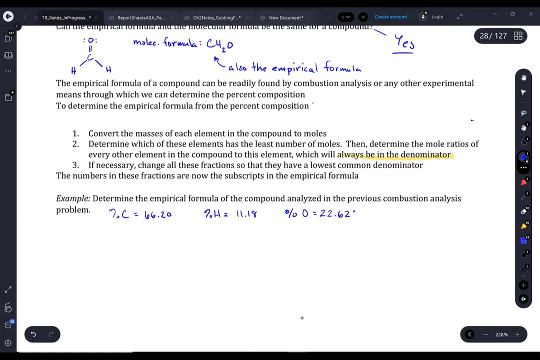 From the previous problem, So some people can remember this for me. So 66.20,, 11.18.. And what was oxygen? 22 point, bless you, 62.. Now, percent composition, if you remember, is an intensive property of a compound. 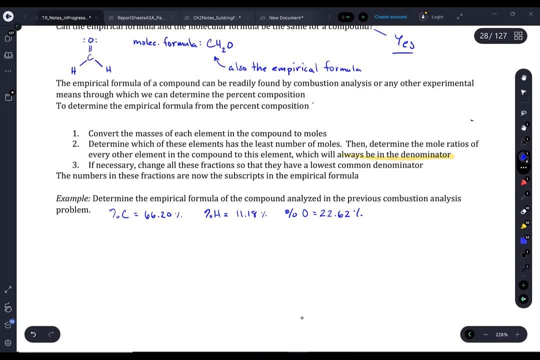 meaning it doesn't change at all depending on the mass or the volume of the compound. It doesn't change. Okay, Now step one says we have to convert the masses of each element in the compound to moles. Now, these aren't masses, These are percent compositions. 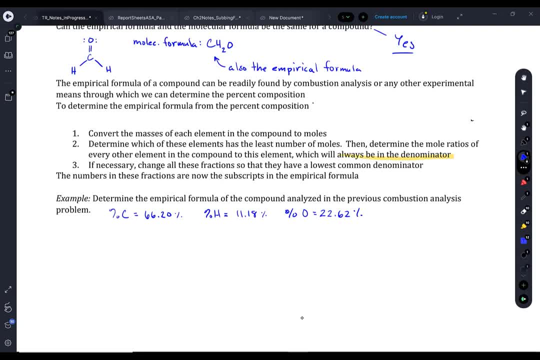 But since this is intensive, you can take the percent composition and convert it to moles. So you can convert the percent composition into moles. You can pick any amount you want. What would be if you're given the percent composition always the easiest amount to pick? 100. 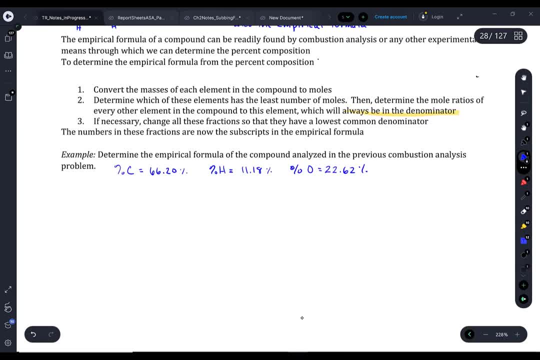 100.. Good, 100 grams. So I'm going to say, assume I have. you don't always have to write this, but I'm going to write it so you have it in the notes. So assume we have 100 grams. 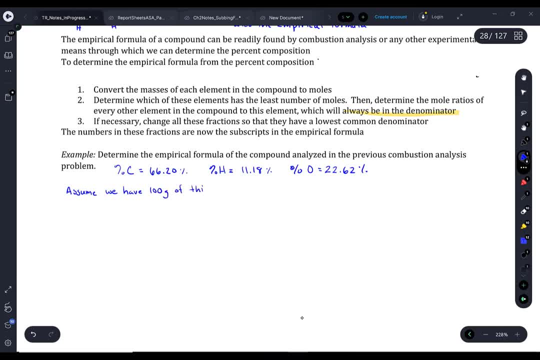 of this compound One more time. That's because the amount that you have is irrelevant. Okay, So I'm going to assume I have 100 grams. So if I have 100 grams, then how many grams of carbon would I have? 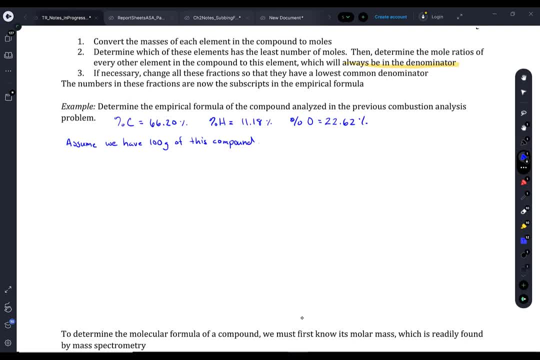 20.. Good, Exactly Because 66.20% of 100 is 66.20.. So for carbon, I have 66.20 grams, For hydrogen I have 11.18 grams, And oxygen, I have 22.62 grams. Be careful that you don't think that O is a zero. 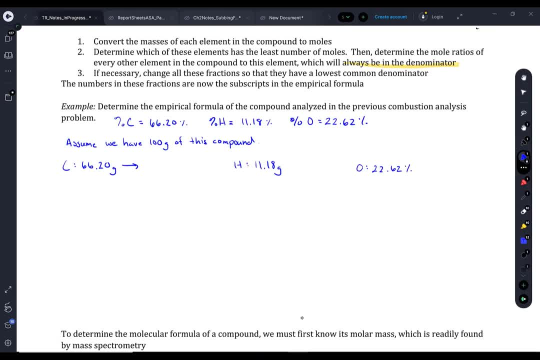 And I need to convert those, as it says in problem one, to moles. Good, Now, if you wanted to create more work for yourself, you could have picked any other mass Like if you want, just prove that, if you'd picked five grams, that you can still do this. 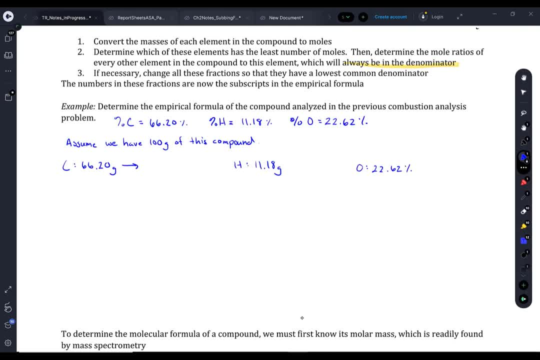 problem. It just adds more steps. You'd have to find out how many grams of carbon you'd have in five grams, All right, So let's convert these to moles, And I'm not going to show my work on this, because you should be able to do that. How do we convert these to moles? You just divide each by. 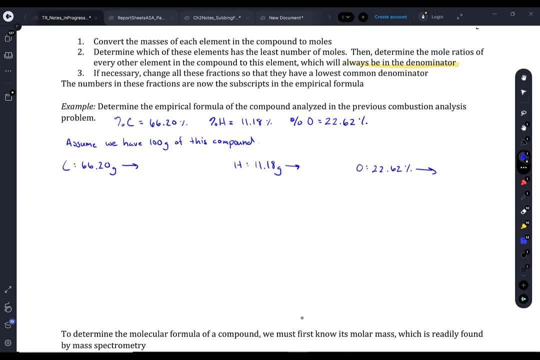 their atomic weight Good. So if I've got carbon, it's 66.20.. I just divide by 12.01.. And that's giving me 5.512 moles. For hydrogen, 11.18 divided by 1.008 would be 11.09 moles. 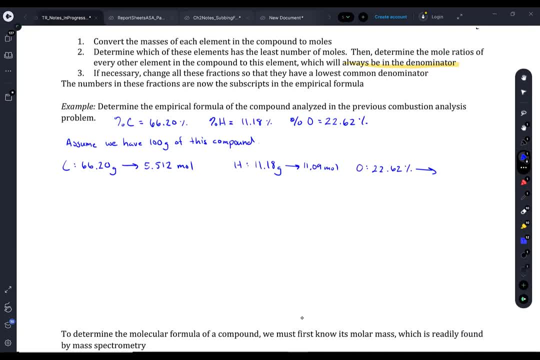 And oxygen: 22.62 divided by 16 gives me 1.414 moles. Now you will always have one less ratio or one fewer ratio than you have elements. So if I have three elements, I will have two ratios. I have to pick which element goes in. 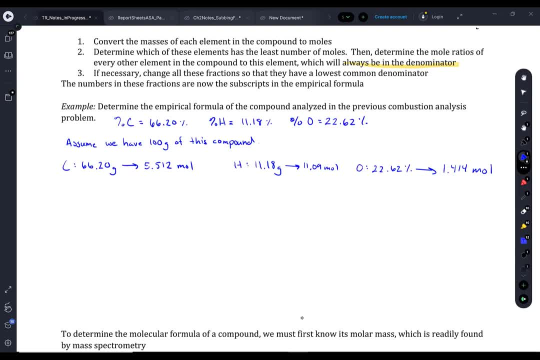 the denominator of all these ratios. And so that's the one with the smallest number of moles. Okay, And so which of these is the smallest number of moles- Oxygen. Good, So what does that mean Whenever you divide these other numbers by the smallest? 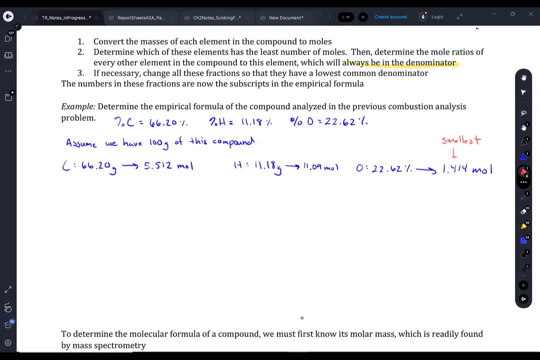 that means you're always going to get a number greater than or equal to one, right, If that's the smallest number, 1.414,. anything else you divide by it will be greater than one. So our ratios, Okay, Are going to be carbon to oxygen. 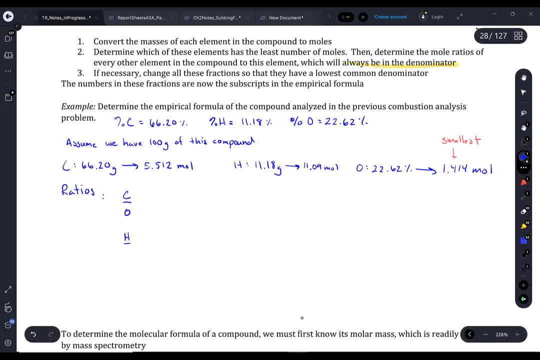 and hydrogen to oxygen. And these are more ratios, because that's what your formula is. It's a ratio of atoms to atoms, which is also a ratio of moles to moles. Good, So 5.512 moles. All right, And then another way we could share it in the think tank or program. So it costs an additional 20.80 to 20.50,ロ. All right, Whether or not you have the general factor or not, That means whether you have all of those Wednesday estad. simplistic perché si? 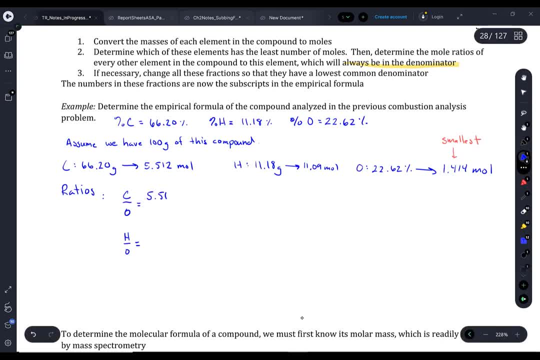 2 moles over 1.414.. Oh, and this problem gives not very good results. I should rewrite it. I'm getting about 3.9-ish, which is very close to this is approximate, right, So 4.. And how do I write 4 as a fraction? 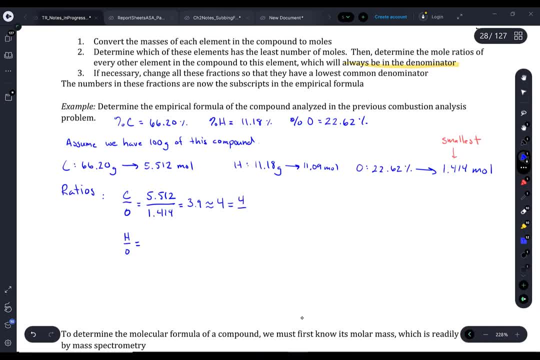 4 over 1, right Good, We always want to end with a fraction. And for hydrogen we have 11.09.. Divided by 1.414.. I'll give you about 8.. Yeah, this is 7.84.. 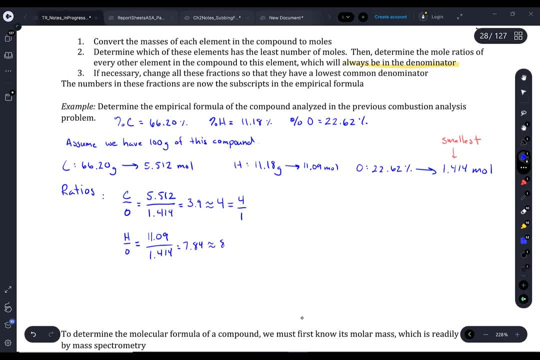 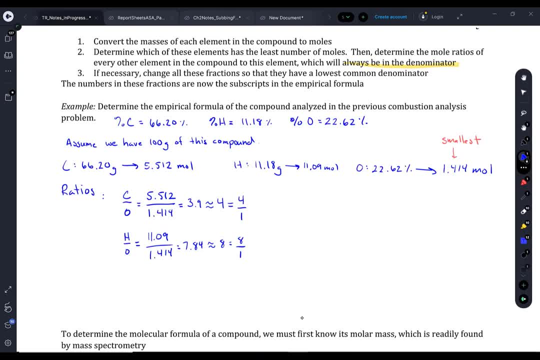 Same digit. Yeah, they're 1.. If they are not the same, then you would have to do step 3, which was get them all to the same common denominator. So, for example, if this had been 8 over 3,, 8 over 1,, if it had been 8 over 3,, then you 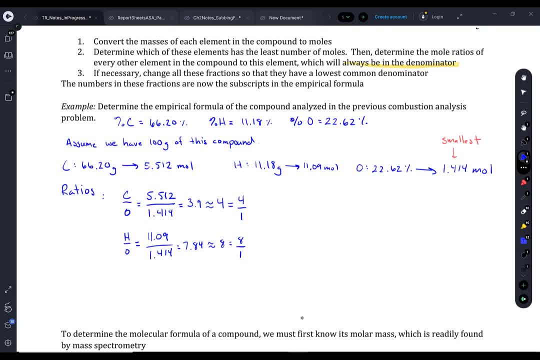 would have to make this one from 4 over 1.. 4 over 1 to what over 3?? 12 over 3, right So, same value, but different denominator. Good, Now we're going to go in the order that I gave you the elements. 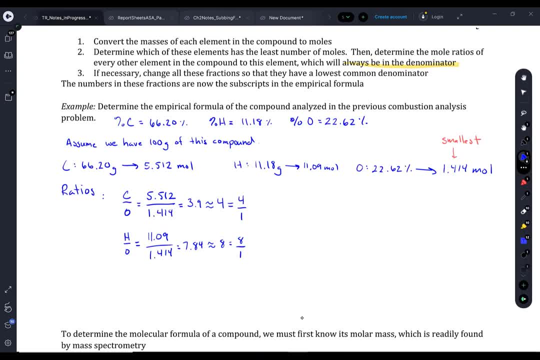 So CHO. So what goes after the C? Good, Do you remember doing this in Chem 120?? Yeah, Combustion analysis was new. So C4.. H, there are 8, because if you look at the fraction H to O And then O will be 1.. 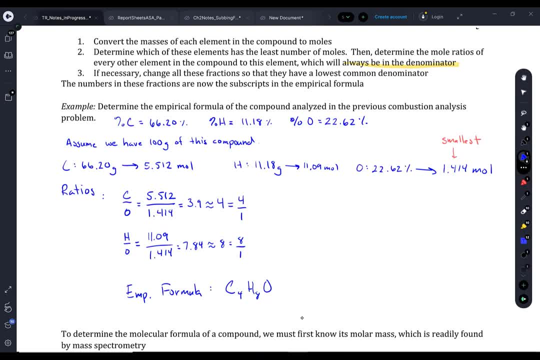 Okay, Now hopefully it's very clear why the denominator now has to be the same. If the denominators were different, then when you get to this stage, what number would you write down If it was a 1 here and a 3 here? you can't. 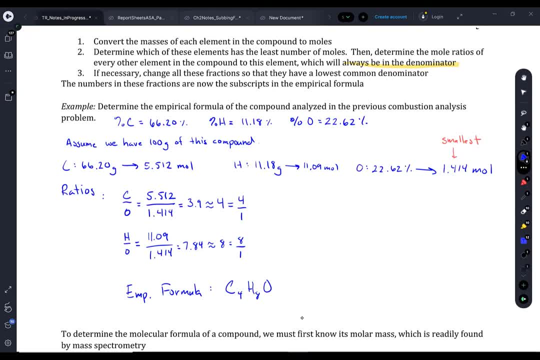 You'll write down 13,, right? No, you can't do that. You have to come down to the lowest whole number ratio. You can all see the screen, right? I can turn these lights off, if it would help, You're fine. 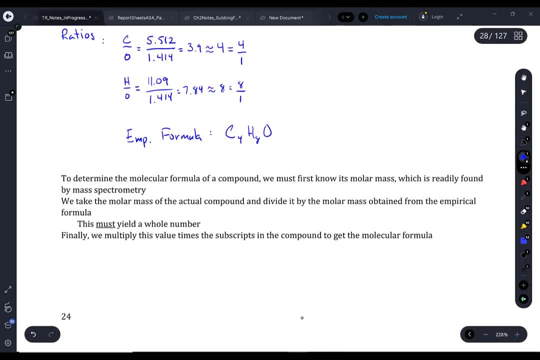 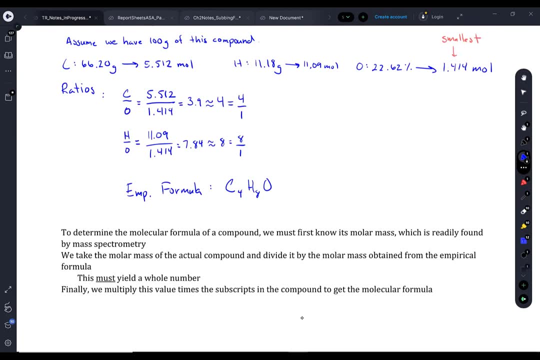 Okay, good, Now I'm only going to give you ratios where the denominator is 1,, 2,, 3, or 4.. I won't give you any others. So let's take a look at this. So let's take a look at this. 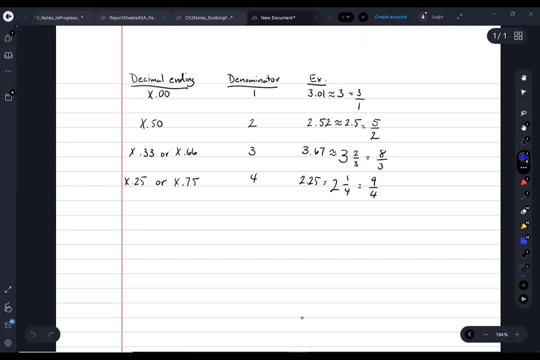 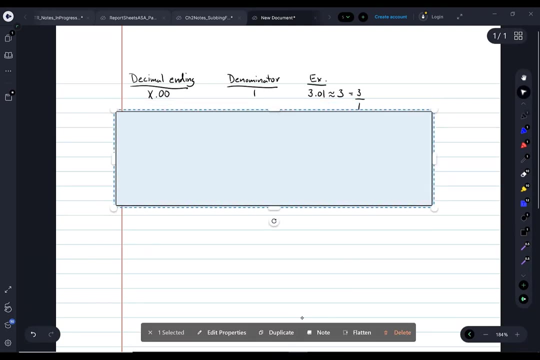 So let's take a look at some potential examples here. I'll wipe these out while I talk about them. Oops, All right, good. So if the denominator is 1, then that means you know when you do the multiple ratio. 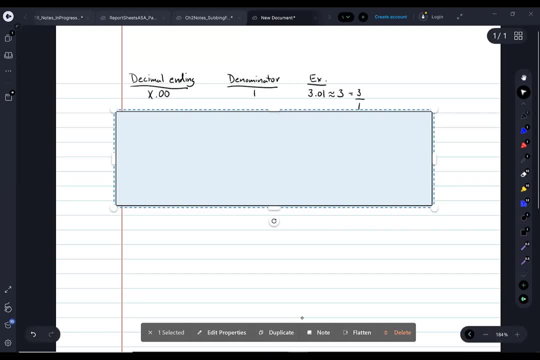 you'll always get something that's close to a number: 0.00.. So like 3.01, 3.00.. Okay, 3.03,, 2.99, 2.97, those are all very close to 3.00, where x could be any number. 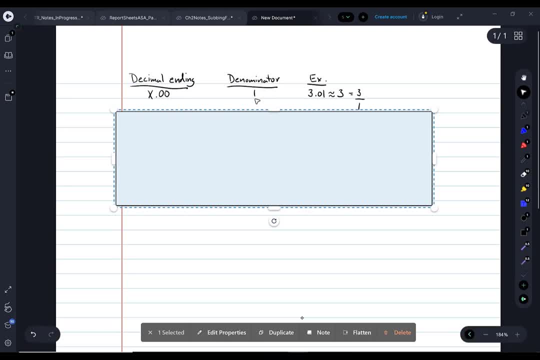 Okay, And so those means the denominators will always be 1.. So 3.01,, for example, is very close to 3,, so that would be 3 over 1.. See, I didn't like my last examples because they weren't like 3.01,, they were like 2.9. 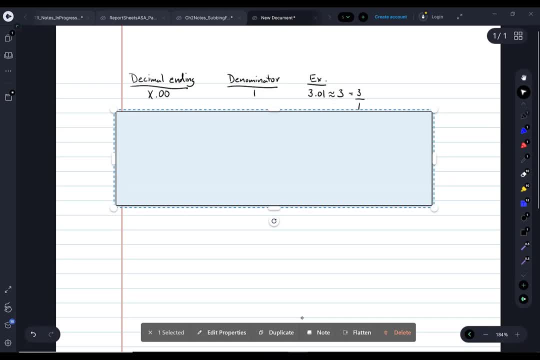 or 2.85,, which is a little farther away than I'd like it to be. So 3.01,, 3.99,, 2.97, those are the ones I'd like the problems to be. Then what would you have if the denominator was 2?? 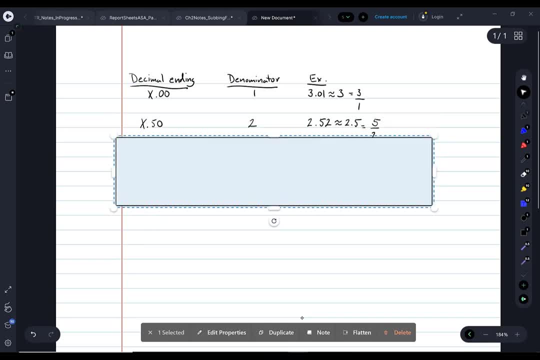 The decimal would have to end in .50, right or .5.. About: These are all very approximate because there's lots of rounding built in. So, for example, if I got 2.52, well, that's a lot closer. 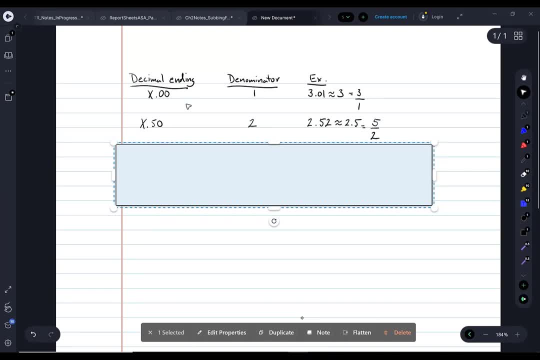 to .5 than it is .0, right. So 2.52 is the same as it's almost 2.5, which, if you wrote it as a mixed fraction, is 2.5, right, And 2.5 written as a. they call this what. 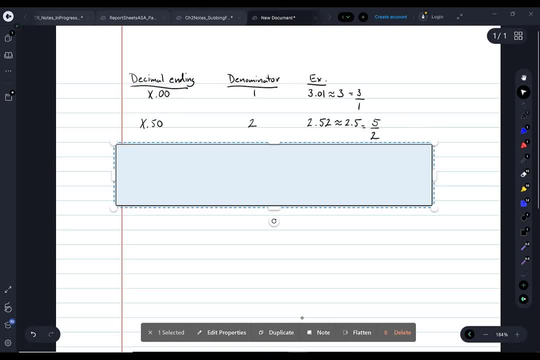 An improper fraction. I hate that term, I'm sorry. Improper is better in my view, So it's very proper to me. 5 .5.. Okay, Is the door? I keep thinking I'm hearing the door people trying to. well, no, they'd bang harder if they tried to get in, wouldn't they? 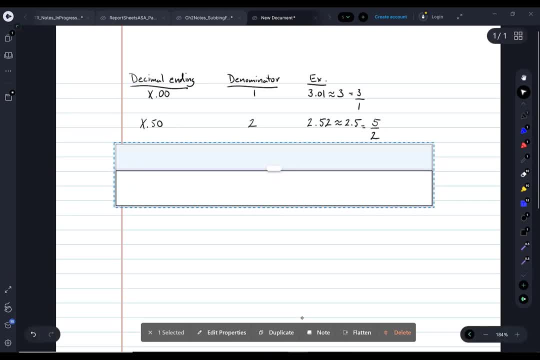 I don't know. I've noticed that when people come to my office hour, frequently I hear and I'm like, well, that's the thing, but I still can't hear you through the door. I mean, you don't have to, you know, but it's like ow anyway. but you get the idea. 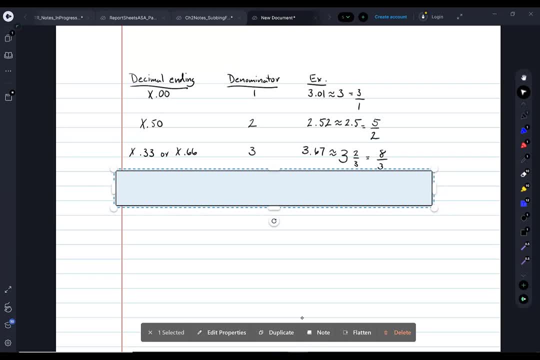 But don't- and I've been saying like a lot today, What, what, louder, louder- I don't know It's just been my hearing's a little off today, Not as bad as my dad. We're constantly yelling at him: get hearing aids, get hearing aids. 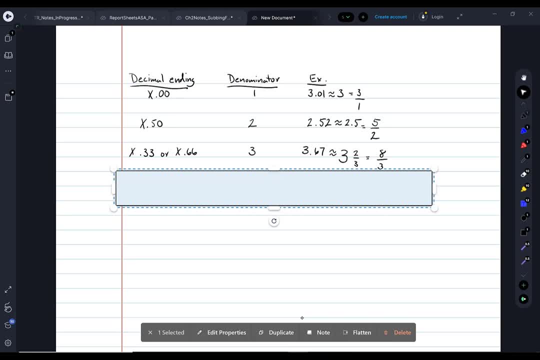 He doesn't want to hear us though. So I think you know my mom has finally realized he just doesn't want to listen to me, So he won't get hearing aids. Anyway, if you get something that ends in about: 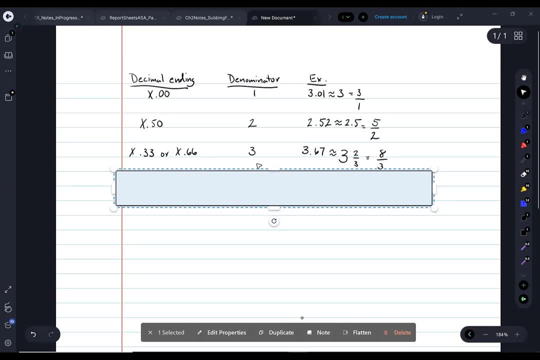 0.33 or 0.66, 0.67, that would mean that the denominator is probably going to be about three, right? So 3.67 is three and two thirds. Yes, And that would be eight thirds. 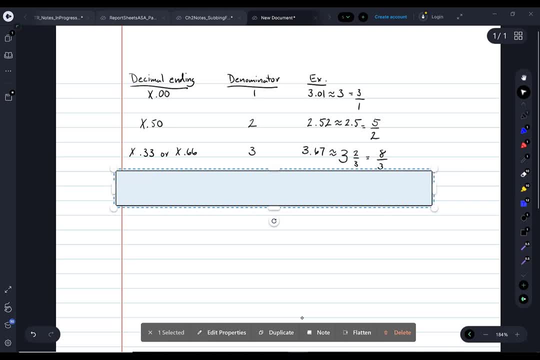 How do you find the numerator here? Three times three. Oh no, this is wrong. Oh, I feel horrid. It's 11 thirds, Thank you. I'll yell at yesterday's class and blame them. No one saw that. 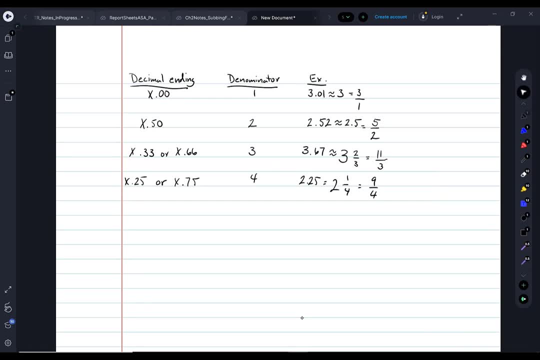 Anyway, and finally fourths, one fourth, three fourths. You can't do two fourths because two fourths is a half. Yeah, good, So anything that ends in about 0.25 or 0.75 would be these: 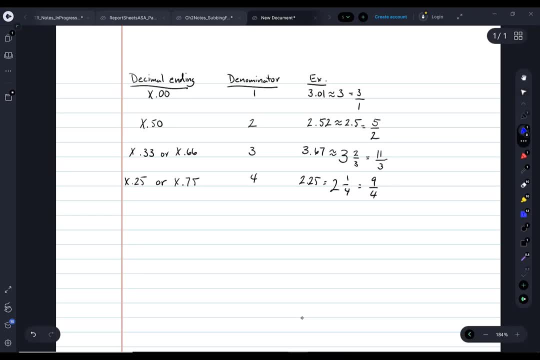 Now, the reason I put up with these- I mean I make these distinctions- is because what if I gave you? So, if I gave you 3.22, this could be approximately what 3.25, by the rules I'm giving you, which is three and a quarter, or 13 over four. 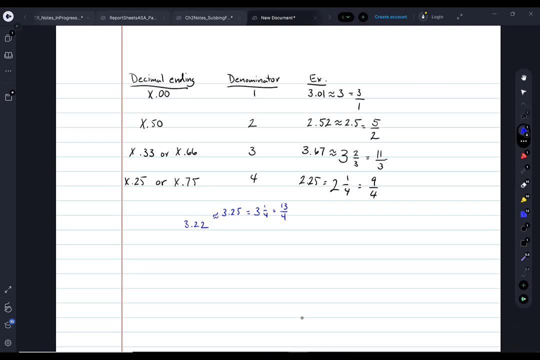 Yeah, But this is also could be very close to 3.25.. So if I give you 3.20, which is three and a fifth, which is 16 fifths. So that's why I'm committing to saying I'm only going to pick problems where the denominator is 1, 2, 3, 4, 5, 1,, 2,, 3, 4.. 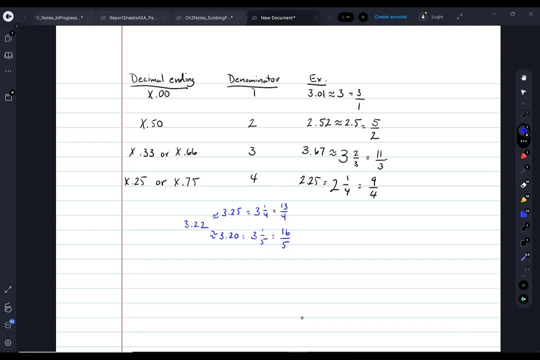 Okay, I think there might be one online where the denominator is a five, but I don't think so Cool, So I will not do this. You will, you'll, you'll, pick the quarter. These are a few of the questions I can't just make up off the top of my head, because I have to find things where the ratios work out. 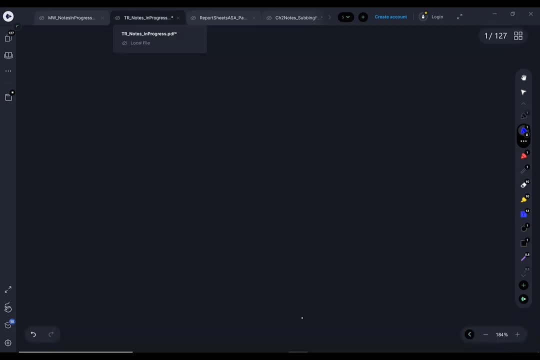 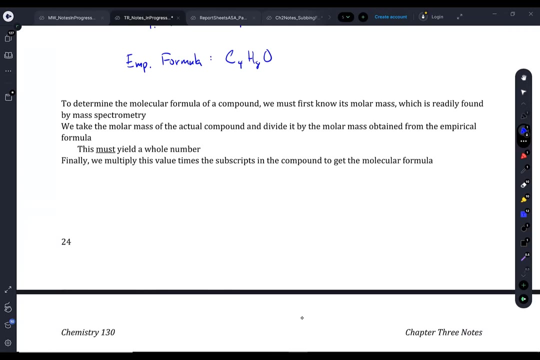 All right, So we all have that, Yeah, Okay, Okay, Now to find the molecular formula, you have to know it's molar mass, Which you could easily find, And so mass spectrometry would give you that molar mass. 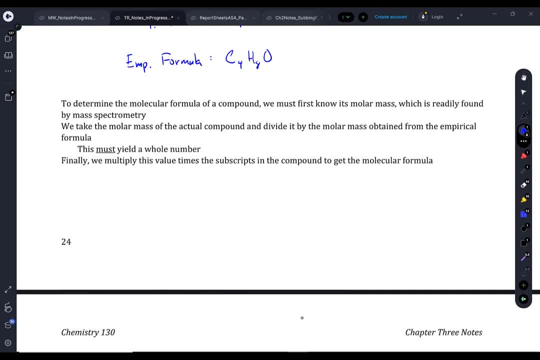 And we can. then what we do is we take the molar mass of whatever compounds formula we found, And it must divide evenly into that molar mass. So again, this is easier seen in a calculation versus doing it in words. Sure, 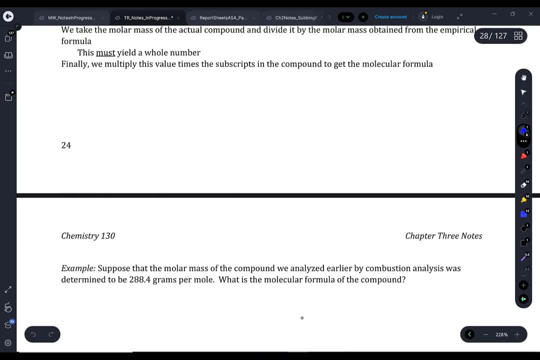 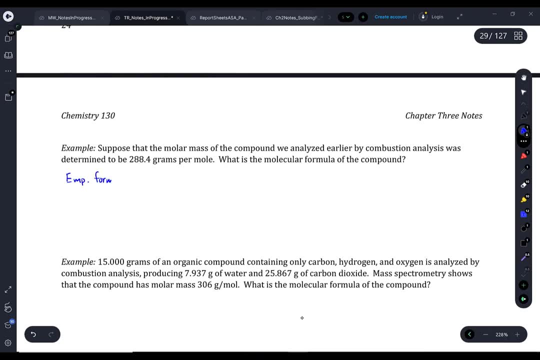 So the last compound that we saw was C4H8O, right, So the empirical formula is C4H8O, And this has molar mass or molecular weight Four times carbon, So four times 12.01 plus eight times hydrogen, 1.008 plus 16 for oxygen. 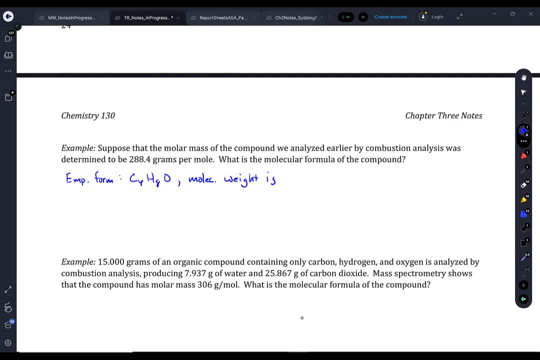 Gives you 72.10.. So this thing called the multiplier is found by just taking the true molecular weight, true 88.4, dividing by 72.10. The molecular weight of the empirical formula, And you should get a whole number here. 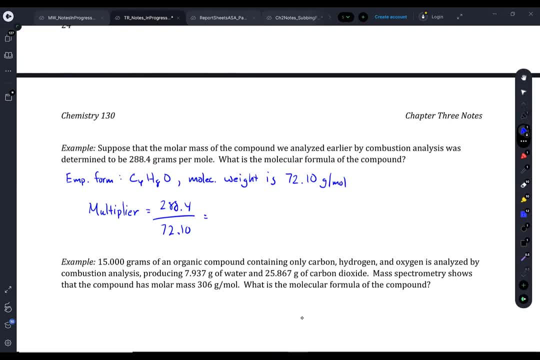 If you're not, that means somewhere you've made a mistake Or something very, very close to a whole number. I got four right on the dot. Is that what you got? Well, pretty much four. It might be 3.99 or 4.0001.. 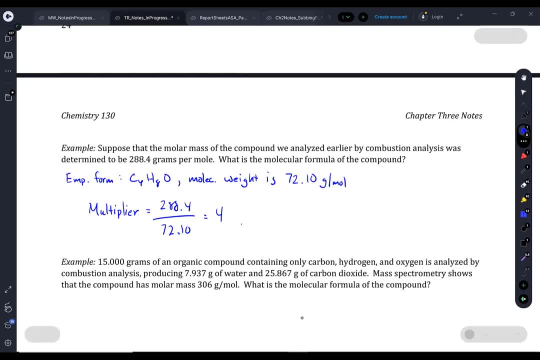 So this means the molecular formula. So it's C4H8.. So four times four is 16.. I'm going to write it the long way. You don't have to do this on an exam. Hydrogen: there's eight of them, right? 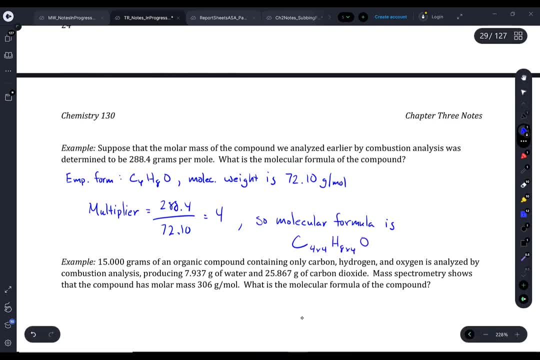 So we're going to multiply that times four. And oxygen, there is one of them, So multiply that times four, which is C16H32O4.. 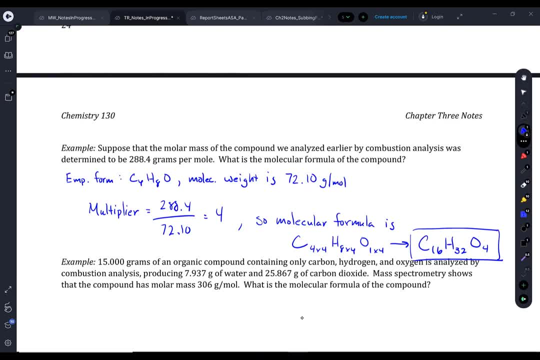 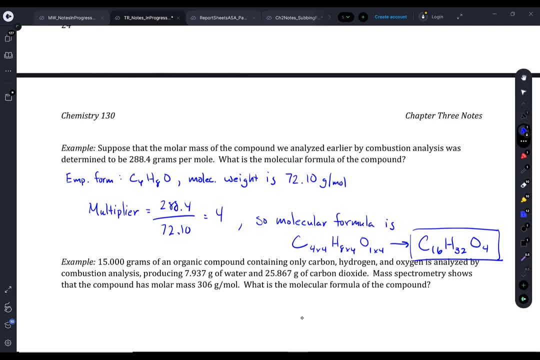 The combustion analysis is nowadays used to confirm. So we would work backwards to say this is really the right answer because you can do it very, very carefully to a lot of significant digits, and so that's how. if you're going to publish a articles saying i made this compound, here's the evidence. i have one of the 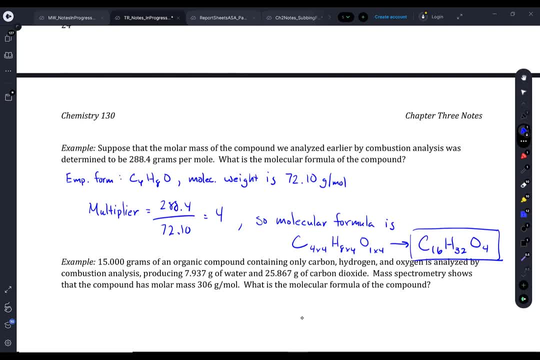 pieces of evidence is you send your compound away to a chemical, to a specialty lab that will confirm that this is in fact the right formula. that's not all, but certainly if that formula is wrong, you couldn't have made the chemical you say you have. okay, good. 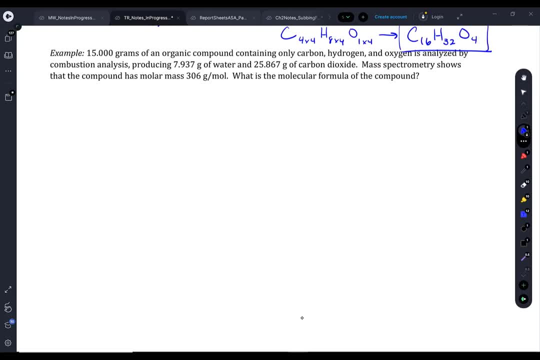 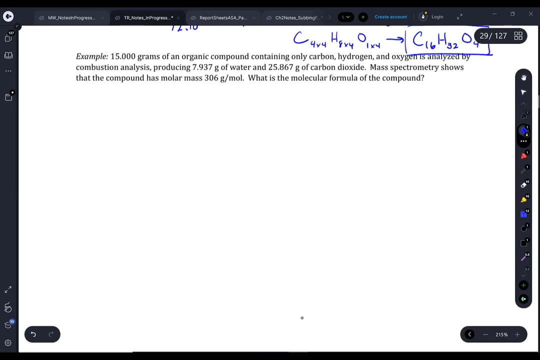 but so this is still more of a classical way of approaching it, the way we learned how to do it historically. all right now this example. i've given you a lot of space right. this example combines all of the last questions. so we have 15 grams of an organic. 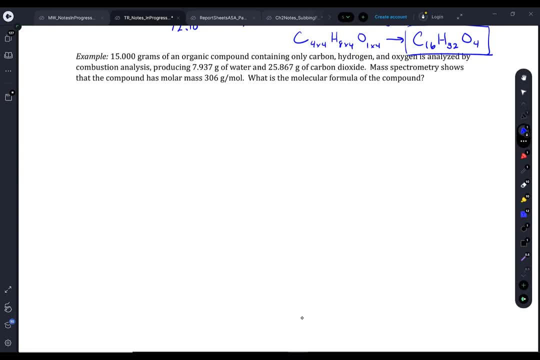 compound that contains only carbon, hydrogen and oxygen. it's analyzed by combustion. analysis gives you this much water and this much carbon dioxide. mass spectrometry shows that the compound has this molar mass. what is the molecular formula? so there's a few ways we could approach this, but i want to go through the same approach. 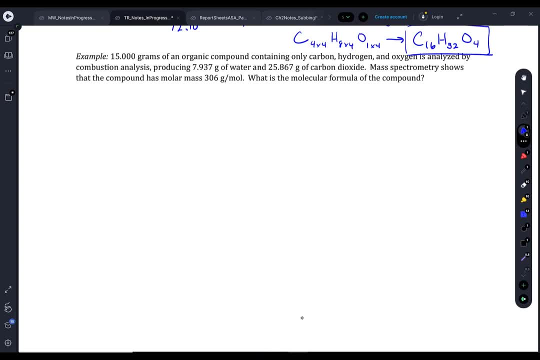 that i did before. so the combustion analysis will first be used. and what does that give me? good, so that's going to be the first part of the problem. first, we're going to use the combustion analysis data to find the percent composition, and it's helpful to remember that the percent carbon 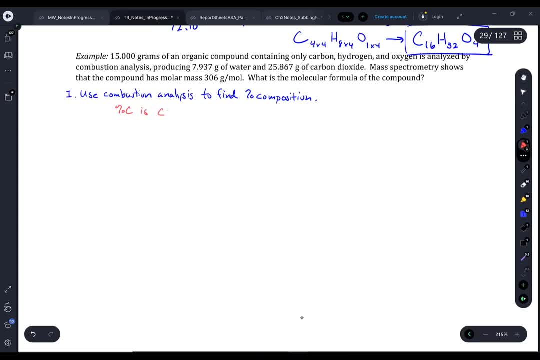 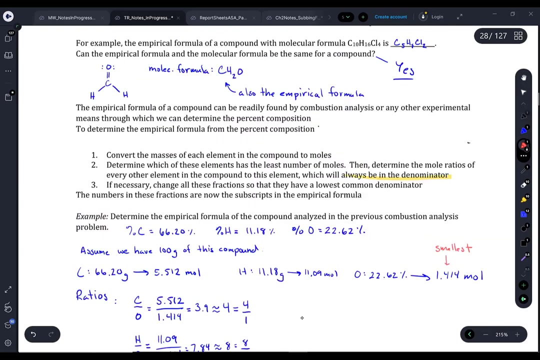 in co2 is something, and the percent hydrogen is something, and the percent hydrogen in water is, i think, 11, something, something all right. so we wrote that down a few pages ago, so let's write this numbers down. so what was the percent carbon in co2? 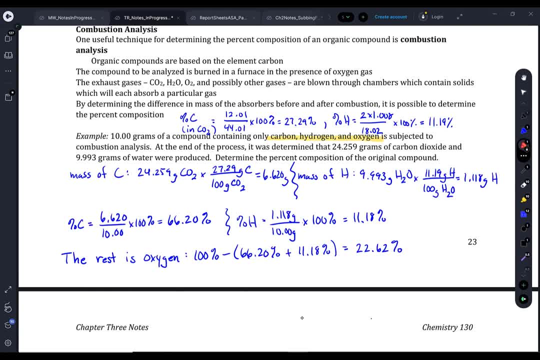 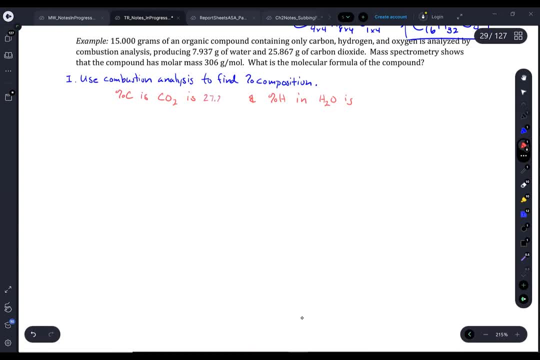 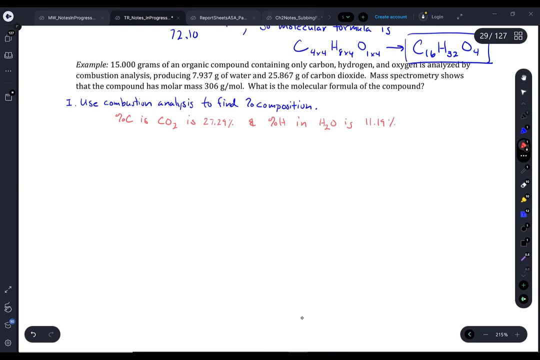 27.29 and 11.19. why are those numbers useful? because what compound do you make in combustion analysis? you make water and carbon. and what's the point of the carbon dioxide? why is it useful? it tells you the amount of carbon in your original sample. 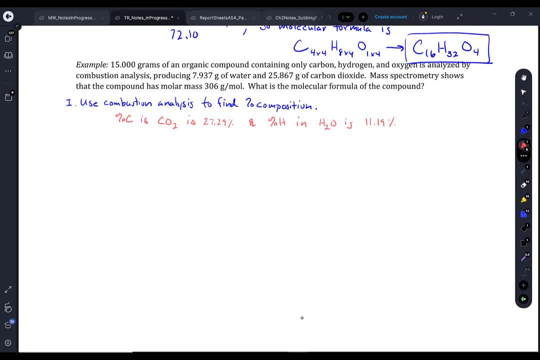 because, remember, when you do combustion analysis, all the carbon in your compound ends up in your mystery compound, ends up in the carbon dioxide and all the hydrogen in that compound ends up in the water. so this will make life easier for us when we're trying to find. 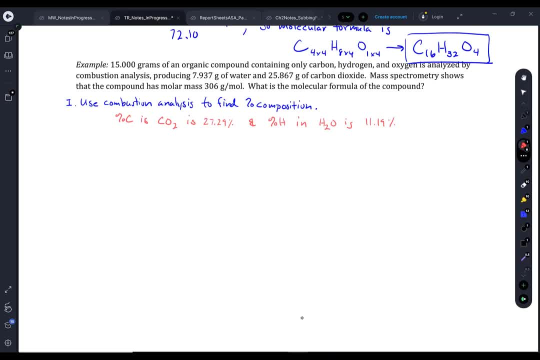 out how much carbon and hydrogen are actually in the compound. okay, so let's find carbon. so let's find the mass of carbon. so we have 25.867 grams of co2, so we just want to find how many grams of that is carbon. so we just multiply by the percent. so for every 100 grams of carbon dioxide there is 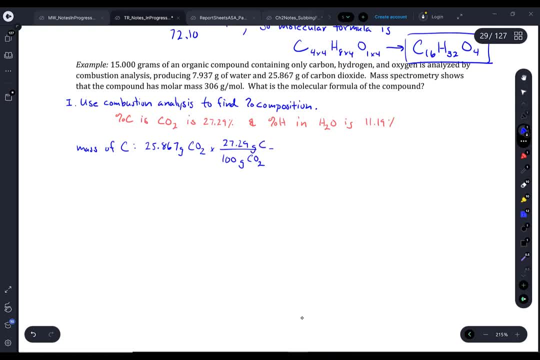 good, 27.29 grams of carbon, or in other words, you're just taking 25.87, multiplying by 0.2729, right, the decimal form of the percent: 25.867 times 0.2729, and so there's 7.059 grams. 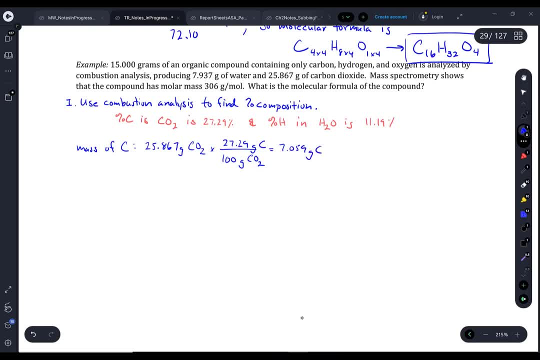 of carbon in the compound. just let me turn that off. wow, lots of spam. that's unfortunate, okay, okay, and then we're going to do the same thing for hydrogen. so i had 7.937 grams of water and multiply that by 0.1119, in other words, 100 grams of water. 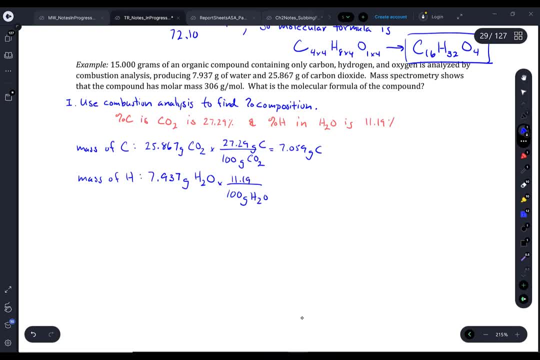 has 11.19 grams of hydrogen, or i'm getting 0.8882, yeah, uh. now i could at this point say that the mass of oxygen is what's left over. right, i'm going to skip that step because i'm just going to go straight to finding. 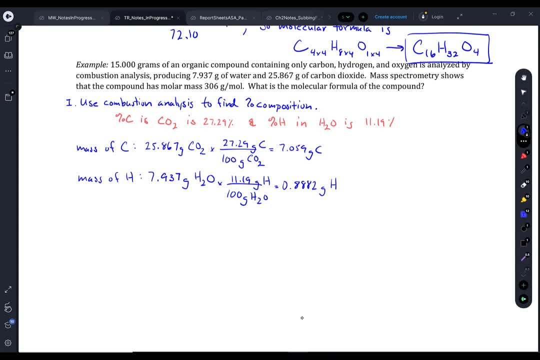 the percents, because i can use the same logic if i find the percent of carbon and the percent of hydrogen, whatever percent is unaccounted for must be oxygen, right, so i'll save myself a step there. okay, so what is the percent of carbon? you might need to read the problem again. not very detailed, but percent of carbon in the compound is. 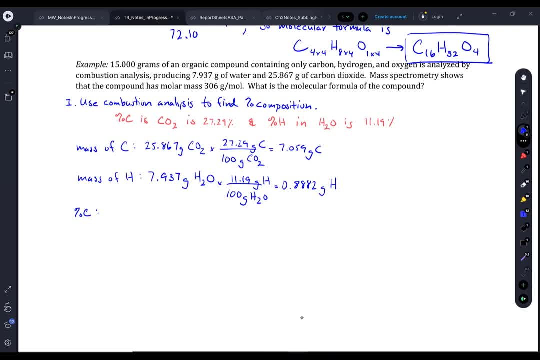 so it's the part over the whole. the part is the 7.059 grams of carbon. what's the whole that's coming from where? no, the 15 grams of the compound. remember, the carbon is coming from the organic compound. so the part is the carbon, the whole is the organic compound, which is 15 grams. 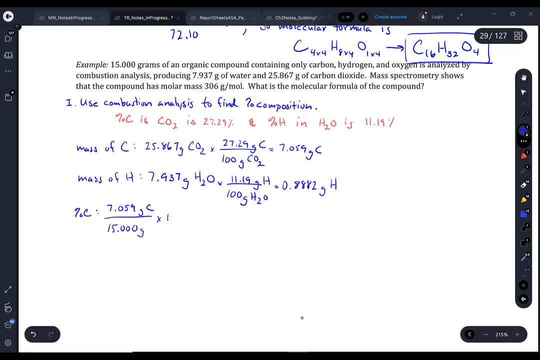 and the carbon is coming from theolder wasта and the whole thing comes from the maximumحد. so for the family size carbon in the compound. let me take a look at my reading back in the video from the quality unitJa所hád家. 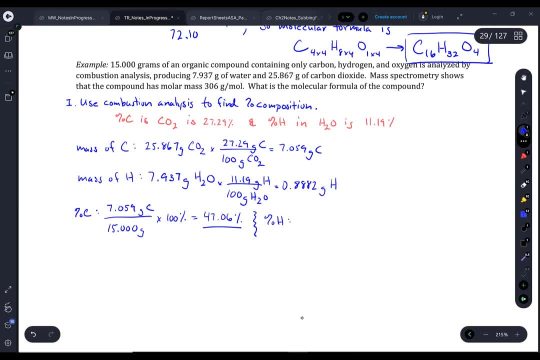 The percent of hydrogen is going to be what? 0.8882 grams of hydrogen over you know what? let me not let me get rid of C, because that doesn't really make sense. Units don't really cancel. So 0.8882 grams divided by the whole, which is 15 grams. 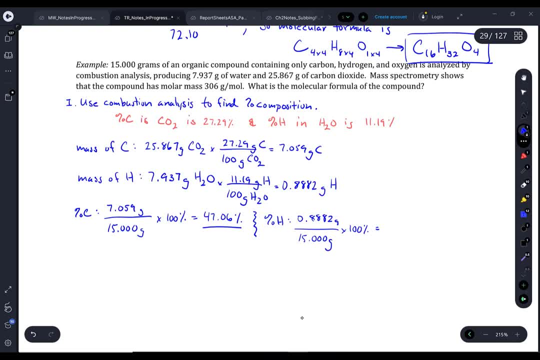 And we multiply that by 100 percent, And so that gives me a quite small number, 5.921 percent. And then what's the percent of oxygen? It's just what's left over. So that would be 100 percent minus the carbon, plus the hydrogen. 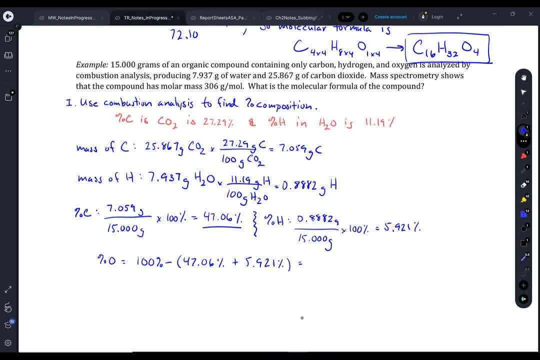 Okay, So 100 minus 47.06 minus 5.921 gives me, I think, 46.. What'd you get? 47.. Okay, Oh, I see why I forgot the five: 47.02, right. 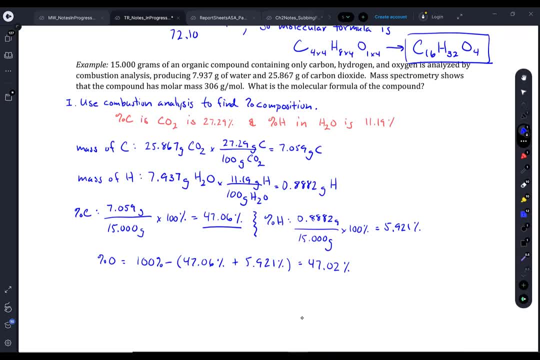 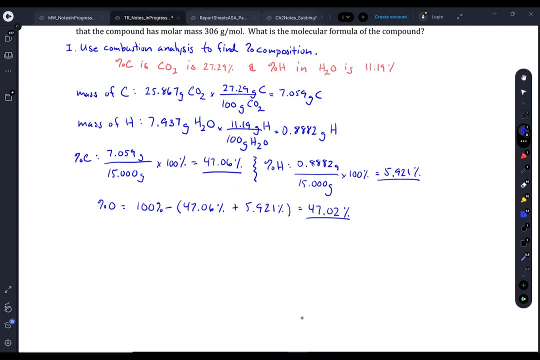 Sick digs, guys, Sick digs. Subtracting that goes to the, The 0.06 hundredths, This goes to the thousands. Good, So I now have my three percentages. So that was step one. That's the new thing that we've learned how to do in this class so far. 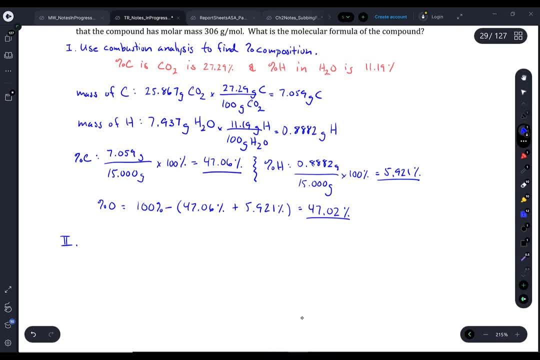 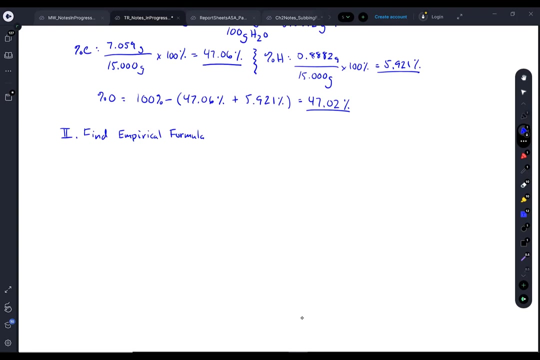 One of them. Step two is: we want to find the empirical formula. Okay, So we've got the empirical formula. We've got the empirical formula. So that's, I think, the first thing we did today. right? So we're going to assume that we have 100 grams of this compound. 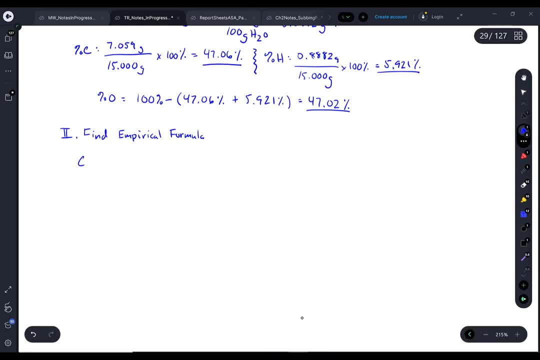 So if I do that means I have 47.06 grams of carbon. So 47.06 divided by 12.01, the molar mass of Atomic mass of carbon and atomic weight is 3.918 moles. 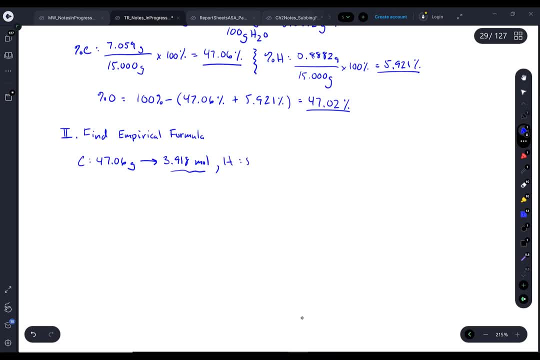 Now we need to do that for hydrogen. We have 5.921 grams, So we're going to convert that to moles. 5.921 divided by 1.008 is 5.874 grams. We have the starting volume. 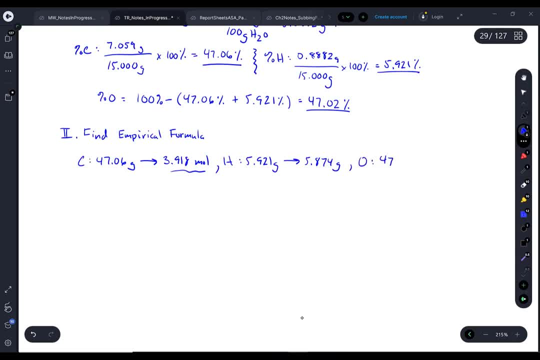 And we need to do that for oxygen. So we have forty seven point zero two grams- Sorry, this is my unit is wrong here. This is moles, And so we're going to divide that by what? Very good, Sixteen off the periodic table, And so that's two point nine, three nine. 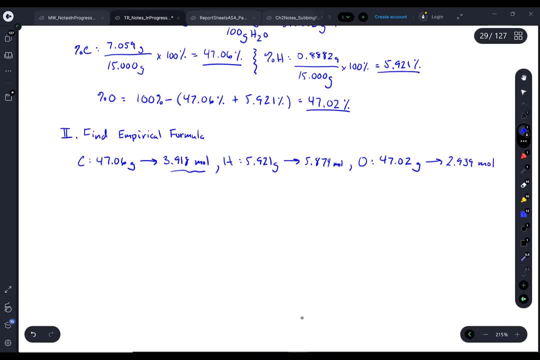 So are we? we're all clear on this step here, right? I just divided each of these masses by the atomic weight on the periodic table for that element. We now identify the. Yeah, this is the least number on here, And that's again. oxygen won't always be, Although it tends to be pretty often. 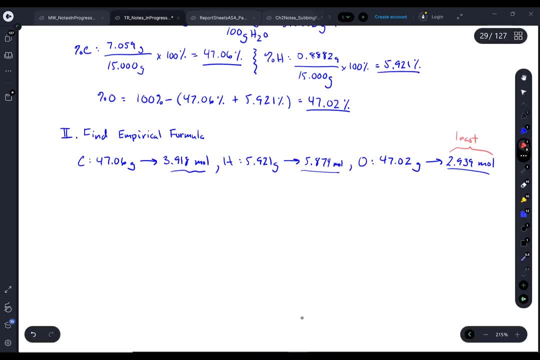 So if this is the least, Then that means it's going to be the smallest number in the ratios. So the ratios will be carbon to oxygen and then hydrogen to oxygen, correct. So carbon to oxygen is three point nine. one eight To two point nine, three nine. 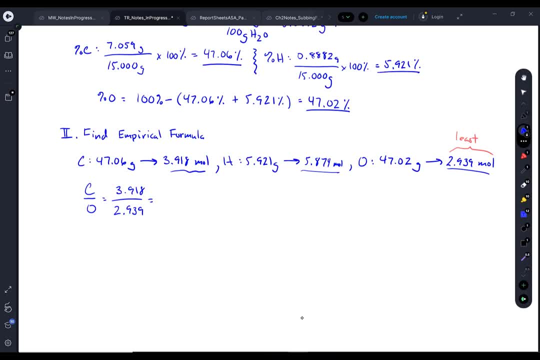 So the ratio is one point three, three. Which is what as a fraction? Yeah, One in a third is four thirds, correct? And the other ratio is, Yeah, hydrogen to Oxygen. good, So hydrogen to oxygen is five point eight, seven, four. 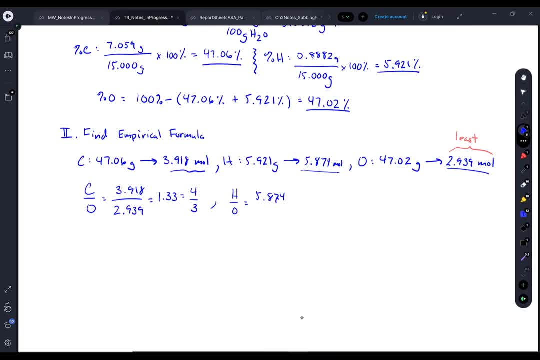 Over two. point nine, three, nine, Which is basically Two, which is a fraction, is two over one, Yeah, Yeah. And now we run into a problem because in the next step, when we go to write the formula, oxygen can't be a three and a one at the same time. 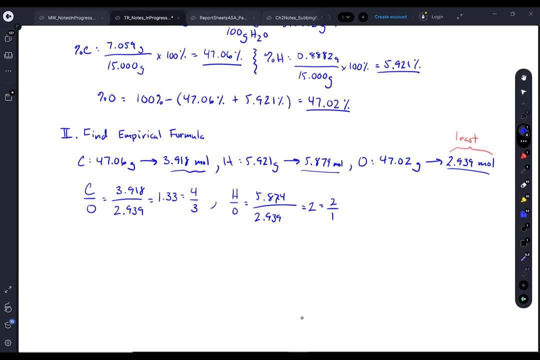 Right. So we need to get this to the lowest lowest common denominator here. So three and one, the lowest common denominator is three. So we'll leave four thirds alone and we'll say two over one is six over three. Good, So again. 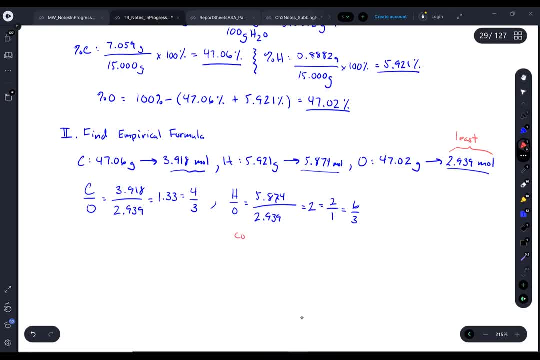 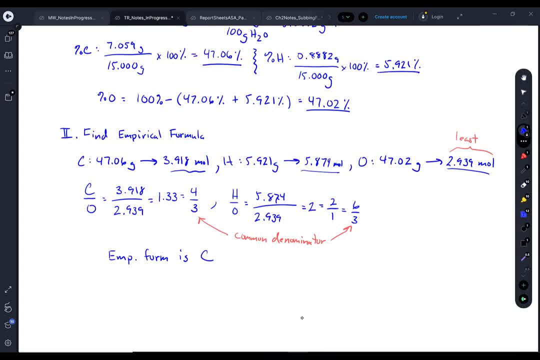 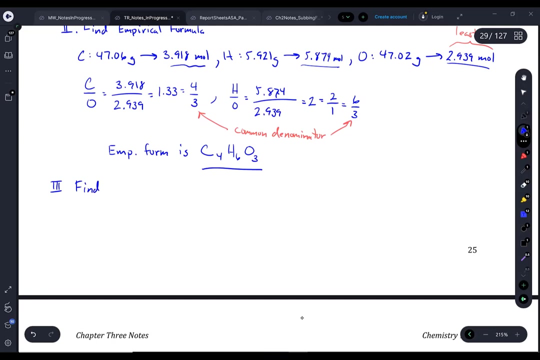 What number goes after carbon Four? Good, So, And then You know. so I chose this from the cork function. So, And then, finally, we want to find the molecular formula. so first we need the molecular weight of the empirical formula. so let's do that. 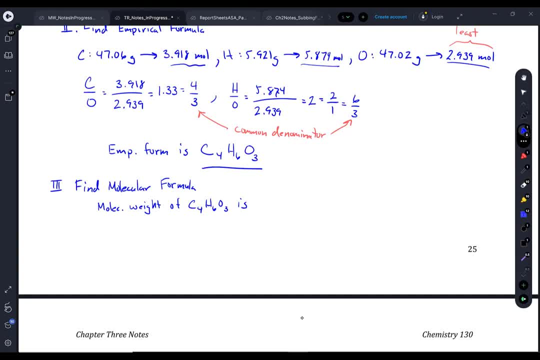 so we've got 12.01 for carbon times 4 plus 1.008 for hydrogen times 6, plus 16 times 3 for oxygen, getting 102.09 and then. and so what were we given? what information were we given about the problem? 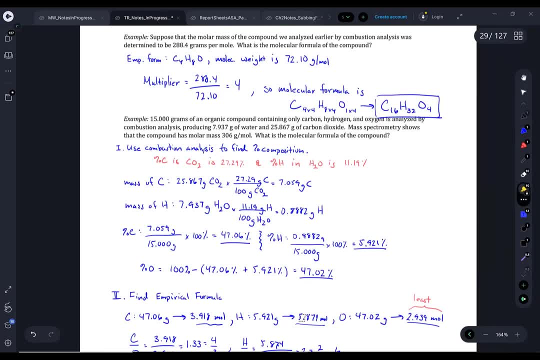 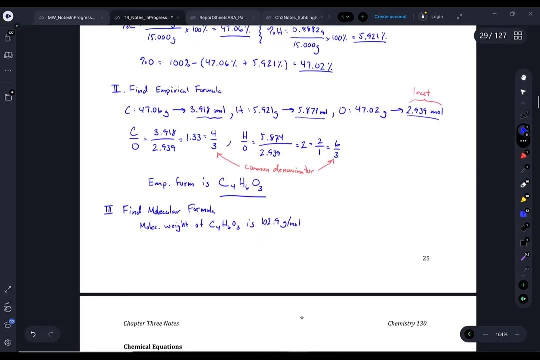 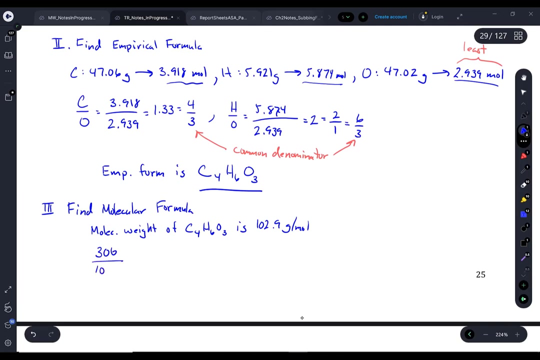 we were given the mass, we were given the mass of water, the mass of carbon, and we were given that it's 306 grams per mole. so that's the last piece of information I need. so so 306 divided by 102 should be very, very close to a whole number. 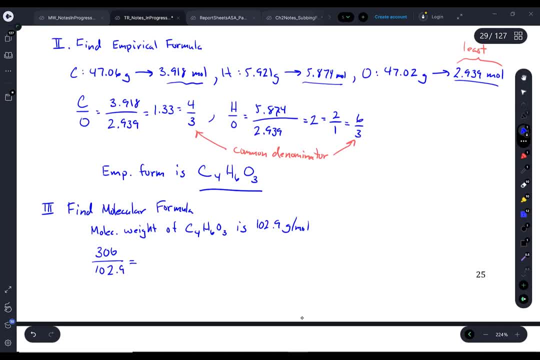 and it is. it's basically 3 right again, if you're getting like 2.7 at that point, that should send warning signals through your mind that you made a mistake somewhere. 306 divided by 102.9- 2.97- that's really really close, right. 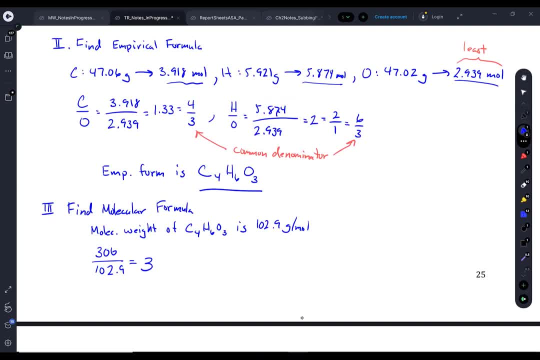 to 3 306. that's really really close, right to 3 102.09. I'm sorry. yeah, you're right. I think it was that we got 306 divided by, because- I'll put it even closer- 2.997. yeah, so it's 3. 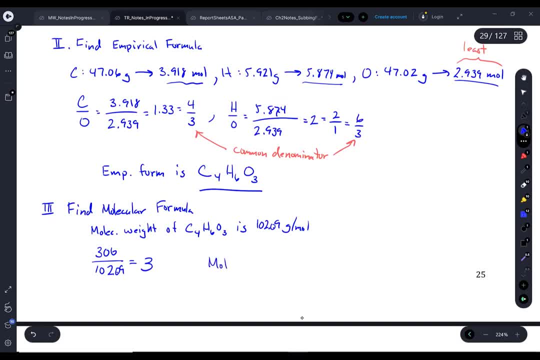 so what is the molecular formula? so what is the molecular formula 0.3? we're just going to multiply all the subscripts by 3 that are in the empirical formula. so C4 times 3 would be C12. H6 times 3 is H18. 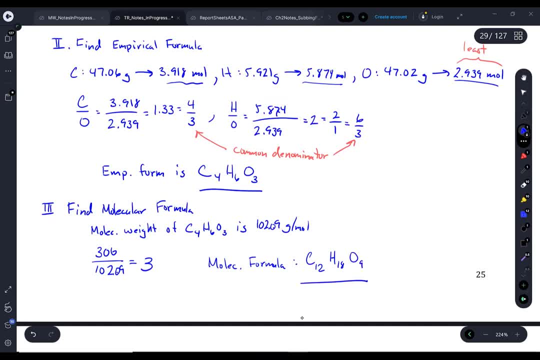 and O3 times 3 is 9, so that's my compound. that's still not enough to find out what the compound is, though right. that's still not enough to find out what the compound is, though right, Right, Because you know there's probably going to be thousands of compounds now with that configuration. 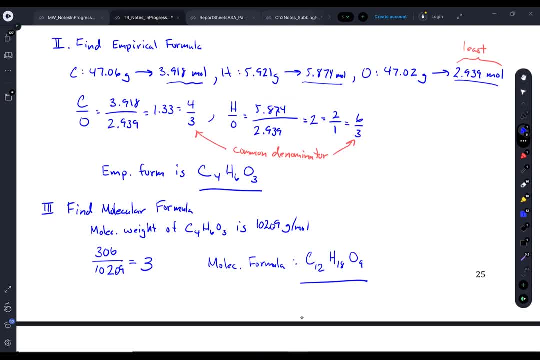 probably not thousands, but tens at least of compounds that have that molecular formula. Yes, that should exist. Sorry, Thinking for a second going. you know that doesn't exist. No, that should exist. OK, Yeah, We all fine, Good. 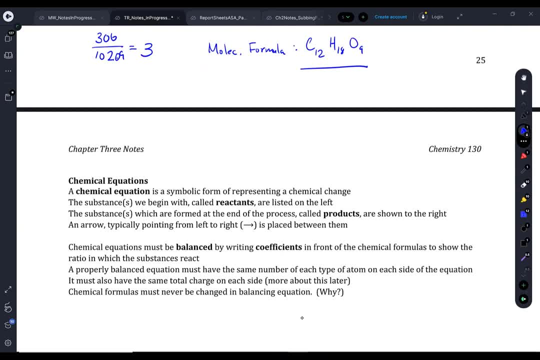 Now in Chem 120, if you remember your Chem 120, this was Chapter 6, except for the combustion analysis, which was kind of new. So everything about moles, that's really been the part that we've been looking for here. 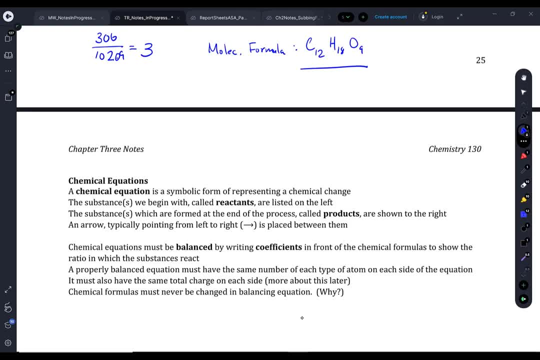 Now we're going to move to a preview of what would have been Chapter 7, which is chemical reactions and chemical equations. In this class, I am not going to go. I'm going to go over balancing chemical equations. OK, you should know how to do that. 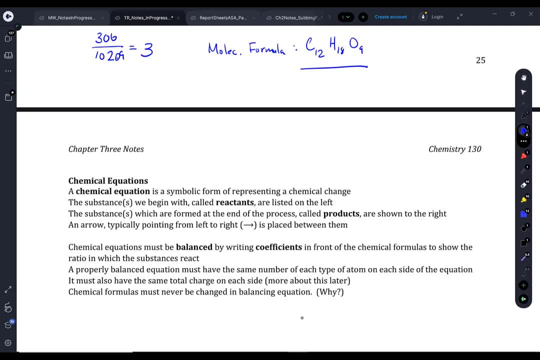 If you can't. if you need practice with balancing equations- there are some in the OWL homework. But under the handout section on the website, click on handouts- There's a worksheet for practice balancing equations. So you should go through and do that. 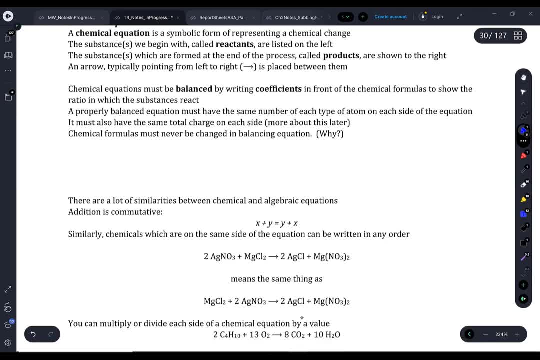 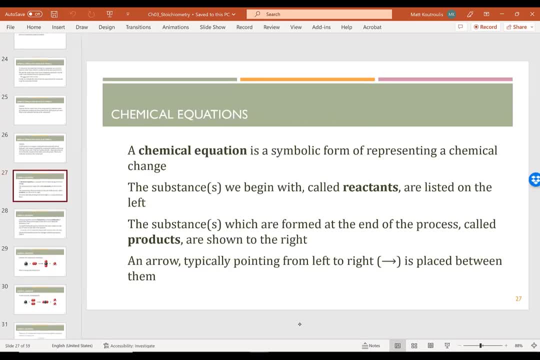 I don't always get them perfectly myself, but it does not hurt. OK, so let's look at some chemical equations here. So it's just the way that we symbolically represent chemical change or a reaction. What we do in a chemical reaction is we begin with one or more reactants. 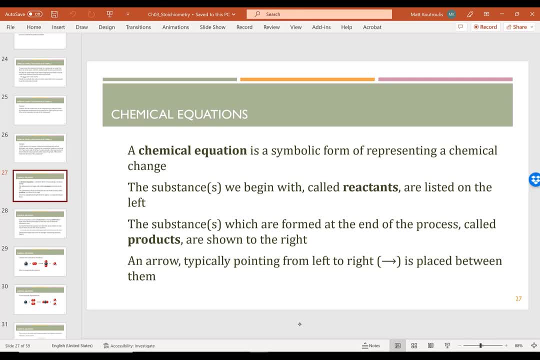 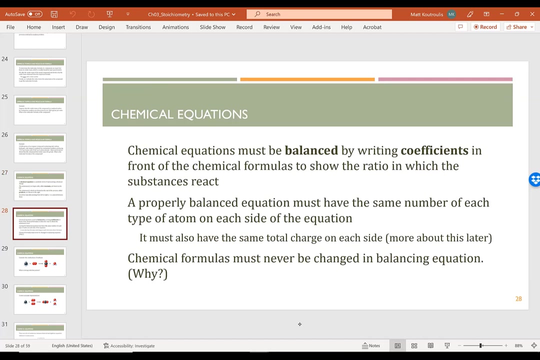 And in a chemical equation we list them on the left typically, And then we make one or more products that we list on the right And in between we put an arrow pointing to the right. So arrow always points towards products. The way we balance a chemical equation is by writing numbers in front of each substance, if needed. 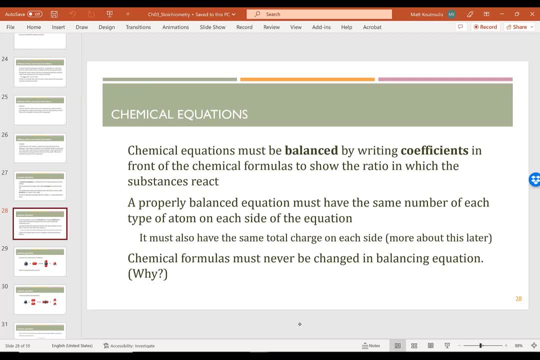 Those are called coefficients, And we will use those in a number of contexts, particularly when we're looking at mole-to-mole ratios in reactions. And The most important issue about this is that you must have the same number of each type of atom on both sides of the equation. 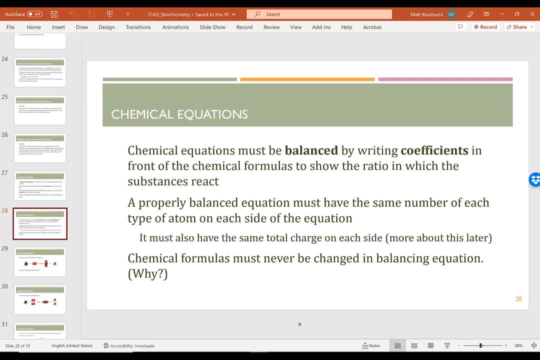 It turns out that you must have also the same total charge. That will be an issue we get into in Chapter 4. that makes balancing equations much, much more involved. It starts to become a 10 to 12 step process, As for right now, since we're not dealing with ions that change their formulas. 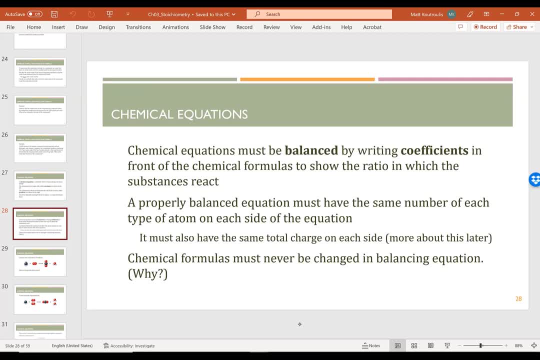 we don't have to worry about that For right now. Now it's critically important that you never change the formula itself in this process. So in other words, if you have CH4 in a chemical equation as part of the balancing, you can't change it to CH6 or CH8.. 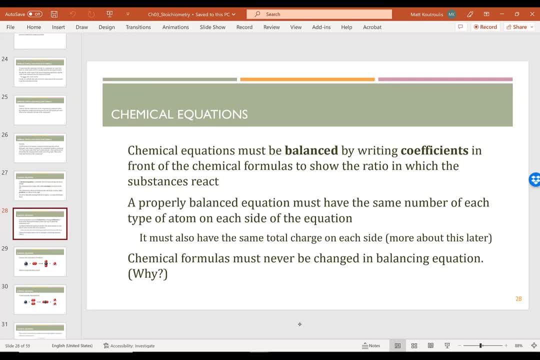 Or you can't change water from H2O to H4O8 or something. You can't do that because then you're changing the formula of the compound. Yeah, yeah, you're changing the compound. You're changing it to something that it isn't. 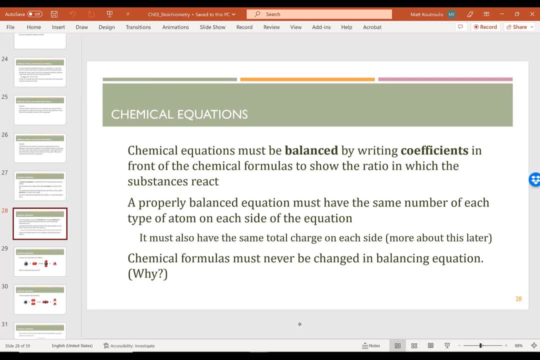 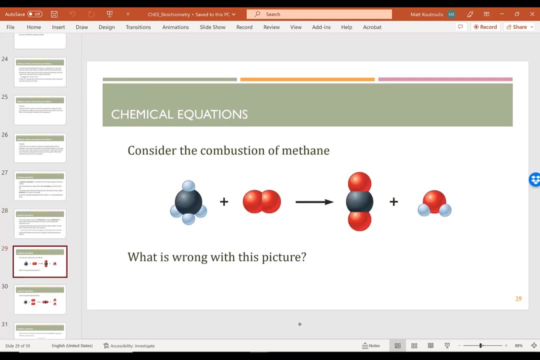 So you may never do that. Why do we balance equations? We must do this as a consequence of the law of conservation of mass right. You must end up with the same number of atoms on each side of the equation, So this is a combustion reaction. 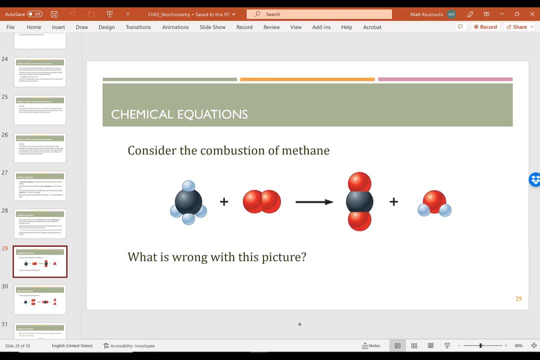 The darkest circles stand for carbon atoms, The red circles stand for oxygen And these, These kind of whitish, bluish ones, stand for hydrogen. So what's the name of this Right here on the left? Yeah, what's its name? 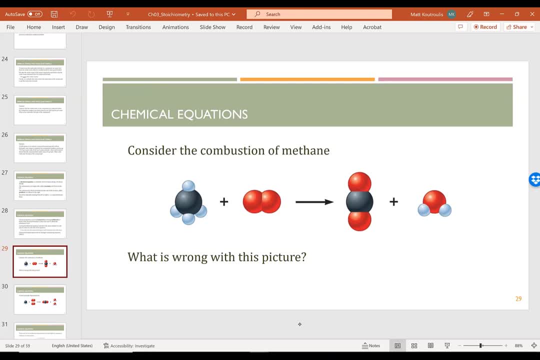 Methane, Methane- good, So methane is reacting with oxygen to make carbon dioxide and water. What's wrong with the picture? as shown, There's more than three oxygens on one side of this, So hydrogen- Is that the right one? 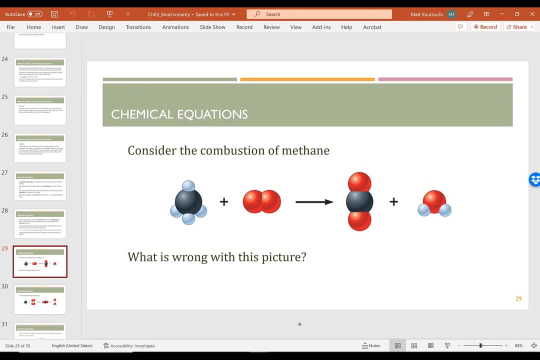 Red ones are oxygens. Oh, there's the three oxygens. There's three oxygens on the right and two oxygens on the left. Yeah, yeah, So there's two oxygens on the left, three oxygens on the right, which implies you. 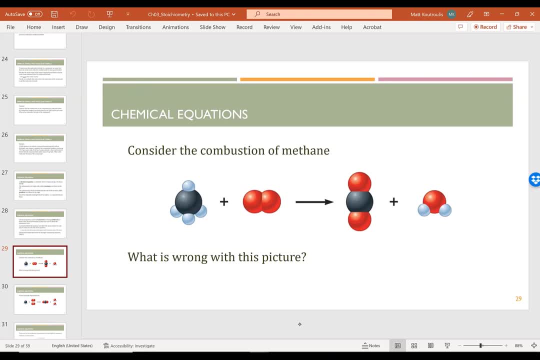 But more articulately if you could. It implies that you have magically created an oxygen atom from nowhere, right? So one sprang into existence that didn't exist. What other problem is there? Lost hydrogen? Yeah, two hydrogens got lost along the way. 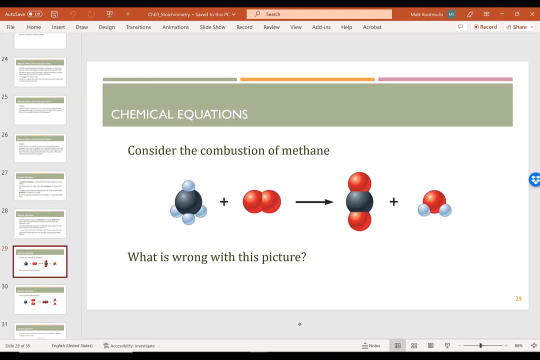 So two hydrogens got together and turned into an oxygen, which doesn't happen, right? So that's how I would interpret that: Two of the hydrogens became an oxygen and they all lived happily ever after, And so that is horribly wrong. 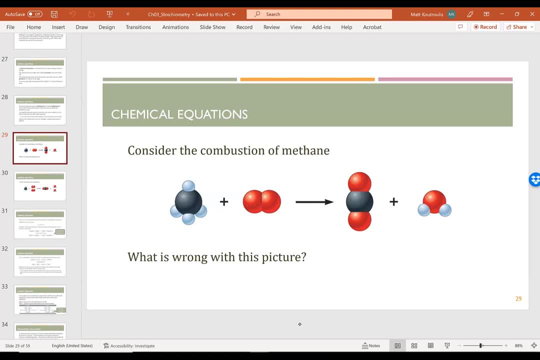 So we need to work out the ratios so that there's the same number of each type of atom on either side, And this ratio would work, Okay, Okay. So what this is saying is: yes, there's a methane molecule, but it now needs two oxygen molecules. 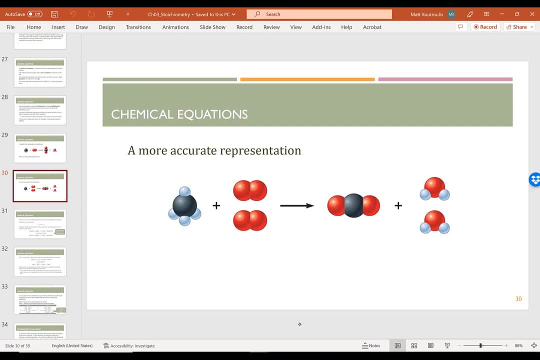 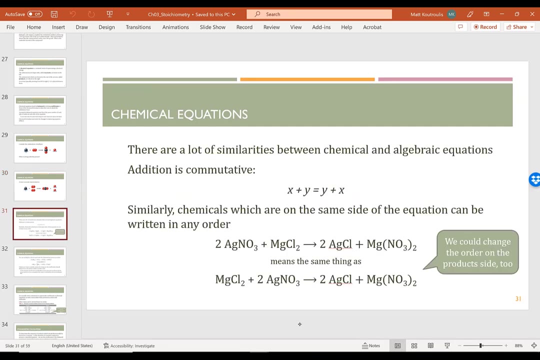 That will give you one carbon dioxide molecule and two water molecules, And now we can account for each atom on both sides of the equation. In other words, the equation is balanced. Very good, Okay, Some general guidelines with chemical equations. We're going to use these, especially starting up in the next lab. 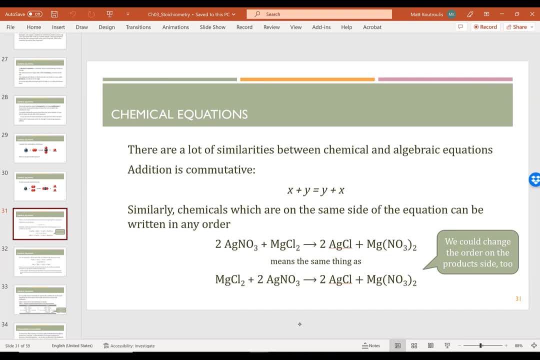 It's important to recall that these behave. They behave a lot like math equations, with the arrow being a lot like an equal sign symbolically. So, first of all, if we remember, in algebra addition is commutative. In other words, x plus y equals y plus x. 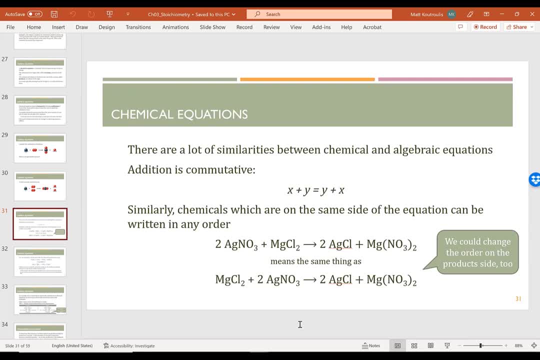 The order doesn't matter. In chemistry. the same is true for a given equation. So as long as you don't move something from one side of the equation to the other, you're okay. So this first equation says two, don't say a, g, n o three. 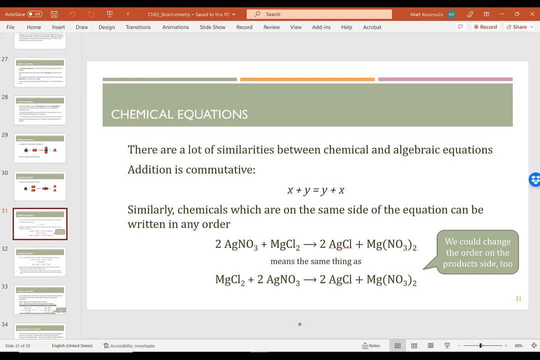 What is that? So two moles of silver nitrate plus one mole of magnesium chloride react, to give you two moles of silver chloride and a mole of magnesium nitrate. Good, Now I could have read it the other way: Magnesium chloride reacts with silver nitrate, right? 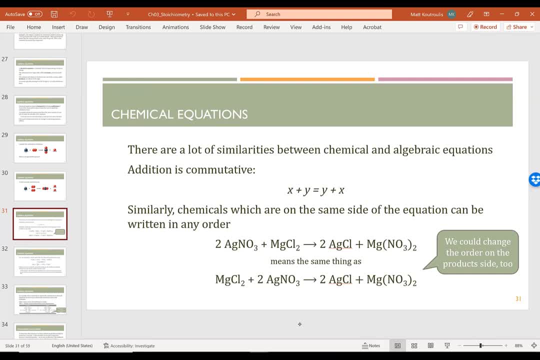 So the way in which I write these is irrelevant. By custom there's some chemicals I use Like I like to. if I'm reacting acids and bases, I always write the acid first. There's no rule saying you have to do it that way. 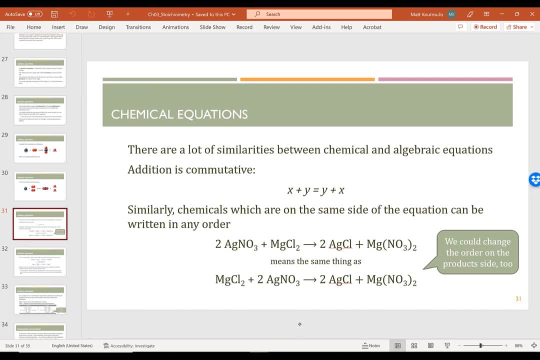 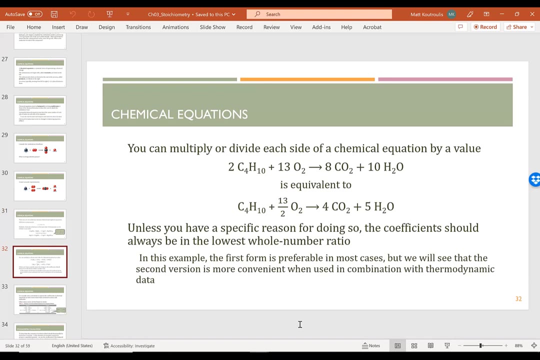 If I'm writing a combustion, I always write whatever is being combusted. plus oxygen gives you CO2 plus water. But if you chose to write water plus CO2, that's no less wrong. So we fine on that Good. You can always multiply or divide each side of a chemical equation by a value. 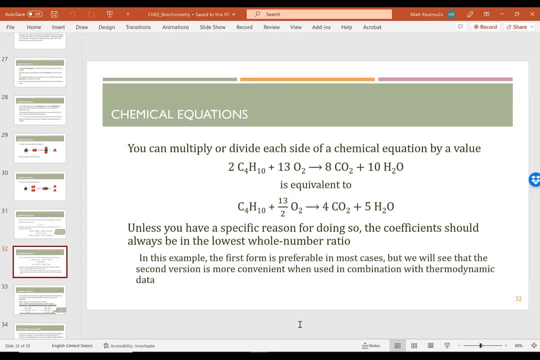 It may no longer appear, though, in a formula, A form which is nice. So if I asked you to write this equation here, the combustion of butane. there's really only two answers that I would accept, And that's the top one and the bottom one here. 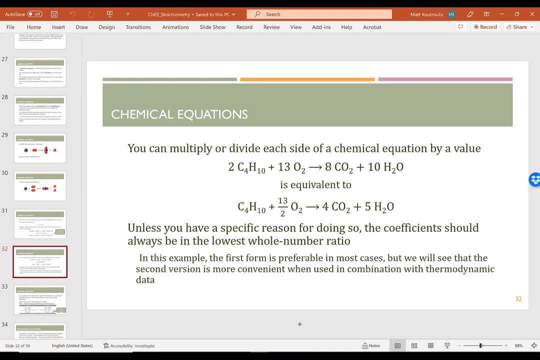 So the first version of this has coefficients 2,, 13,, 8,, 10.. 13 is a prime number, right, So it has no common divisors other than one. So this is in the lowest possible ratio. 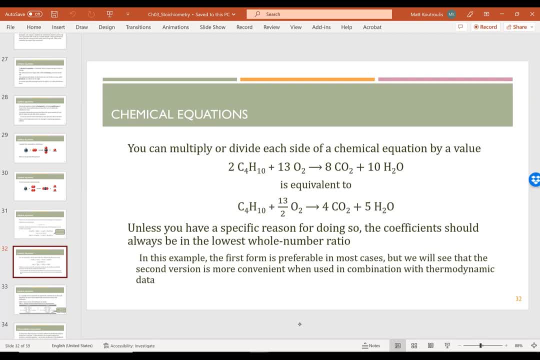 So I wonder Everything to be in the lowest whole number ratio, if I can Now. if I want, though, I could divide everything by 2. And that would give me this balanced equation here. The only issue, though, is that introduces a fraction into the problem. 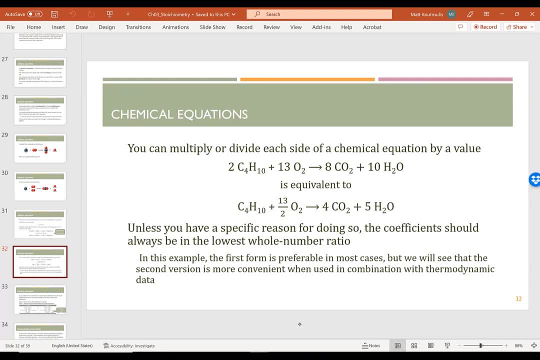 I only make mention of this because later on, when we start getting into thermodynamics and we start saying: you know how much energy does this produce For a lot of chemicals, the amount of energy that it takes to burn some that is given off and something burns is expressed as per mole, per 1 mole. 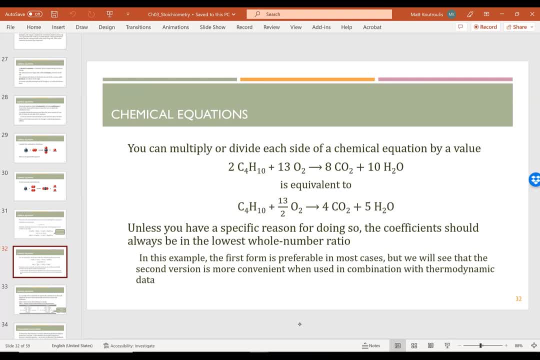 And so which of these would technically be easier? if you're talking about butane, C4H10,. if you're saying how much heat is given off per mole, The bottom form, right, Because the top form is for 2 moles, okay. 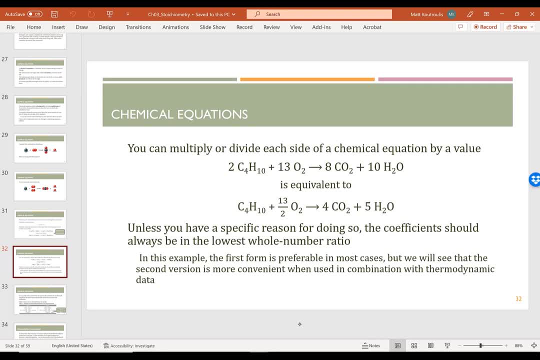 So it means you don't have to take into account the 2 being there, So there will. There will be some times where we have to use fractions, but they are rare. Should we be scared of fractions? No, they are our friends. 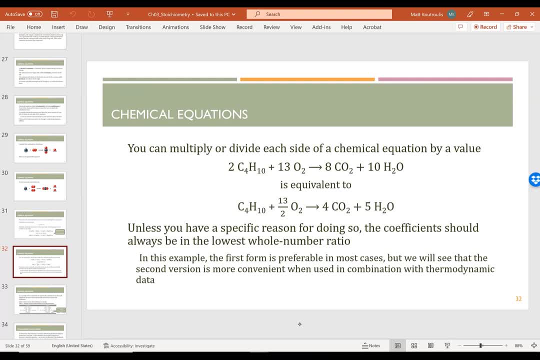 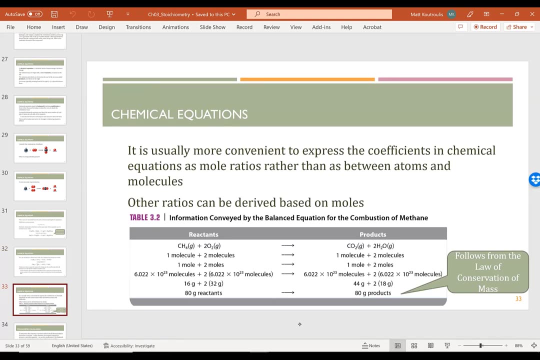 But if you use those in a calculation, don't write the fraction, Write it as a decimal. 13 halves is what? 6.5, 6.5, right, Yeah, Good, And rather than saying atoms to atoms, 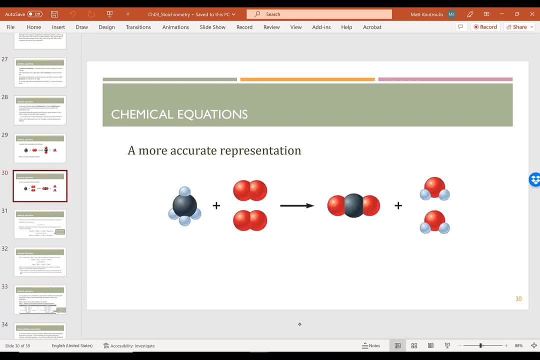 Like we did here, or molecules to molecules. that's really inconvenient. So instead we're going to say moles most of the time. Now I can't say grams, right, Because the mass of all of these things is different. 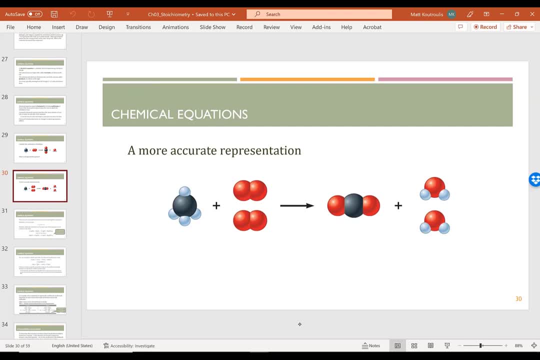 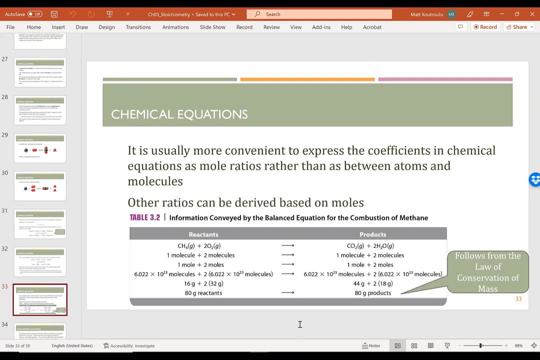 The mass of methane is A mole of methane is different from the mass of a mole of oxygen, et cetera. So the book gives you this table that shows you all, technically, the different ways that you could write these. So we'll. 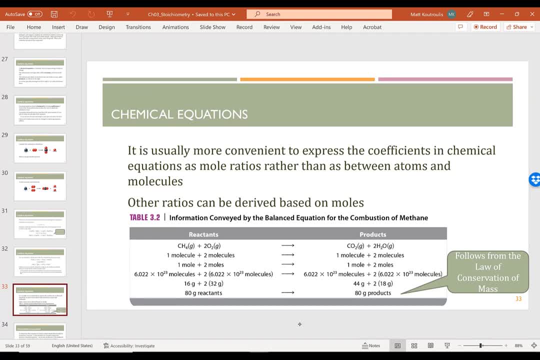 We'll normally write it the way on the top, But we will understand it as the third way. A mole of CH4 plus two moles of oxygen gives you a mole of carbon dioxide and two moles of this. Using Avogadro's number, we could break that down into numbers of molecules. 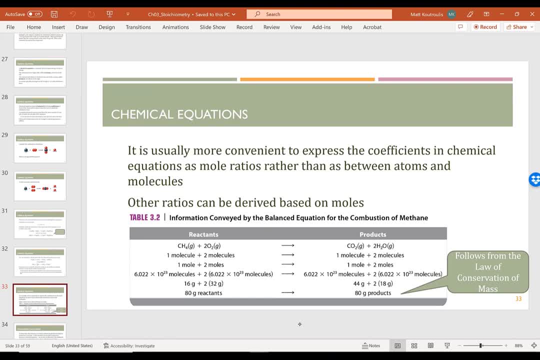 And we could break that down further to grams if we wanted to, But we don't write grams in front. But ultimately, you notice, if you do convert all this, you get 80 grams of reactants, giving you 80 grams of products. 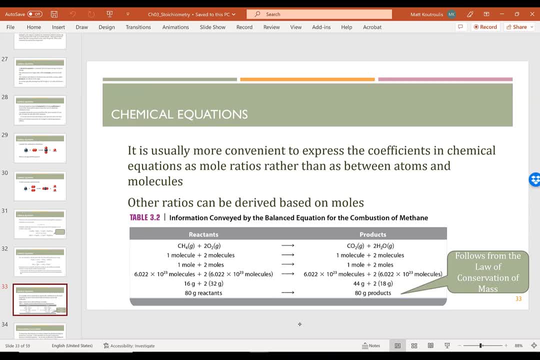 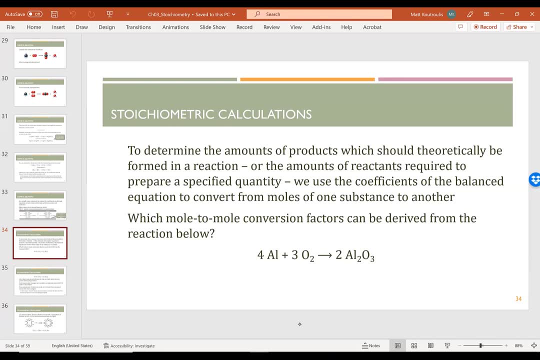 Is that what we would expect? Yes, Good Conservation of mass says that that's what we should get. All right. So if we want to figure out the amounts of products that should be produced in a chemical reaction, Or, going backwards, if we know the amount of products, figuring out the amount of reactants, 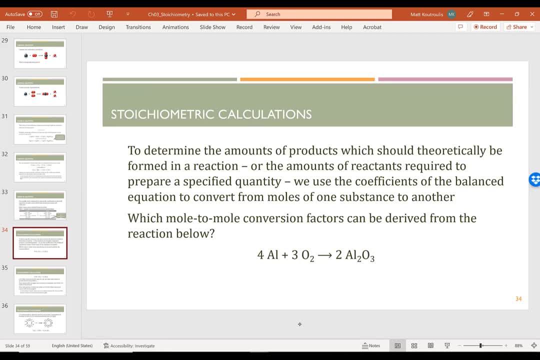 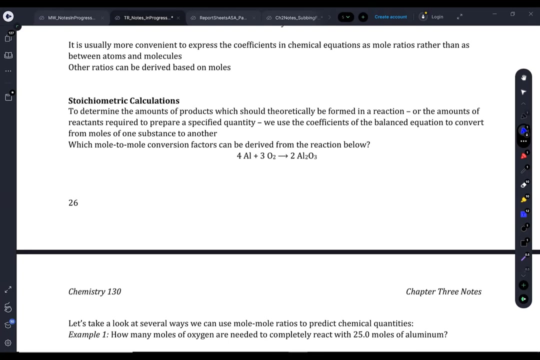 We can use the balanced equation to come up with the ratios that everything reacts in or is produced. So here, for example, is the reaction of aluminum with oxygen gas to make aluminum oxide. I can get from here six ratios. For example, I could get for every four moles of aluminum. 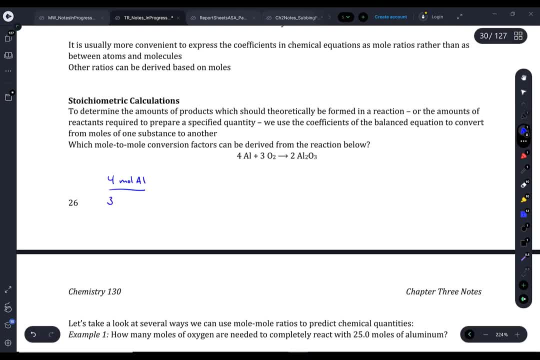 There must be three moles of oxygen For every four moles of aluminum that I produce. for every four moles of aluminum, that would correspond to two moles of aluminum oxide. For every three moles of oxygen, that's related to two moles of aluminum. 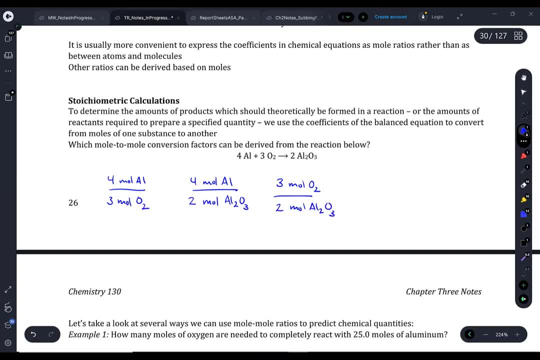 Okay, And then there's three more. They would be the reciprocals of those Right. So this would be used to convert moles of oxygen to moles of oxygen. So this would be used to convert moles of oxygen to moles of aluminum. 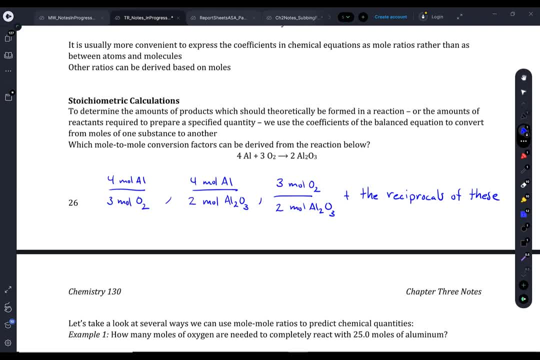 The reciprocal would be used to convert moles of aluminum to moles of oxygen, et cetera. So all this is telling me is- and it's very powerful: I only need to know the amount of one of these to find the corresponding amount of all other chemicals. 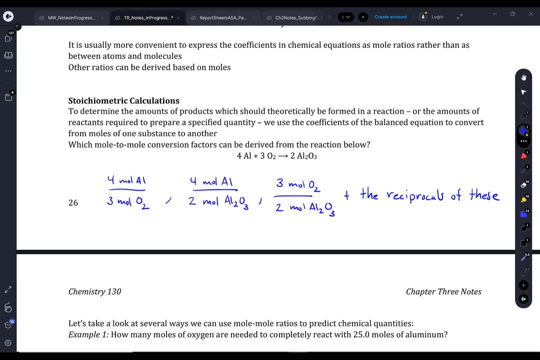 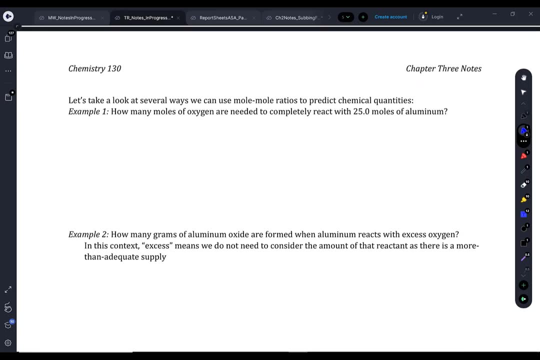 Right, Because I can use the mole ratio. Any questions, Any issues with that? No, Okay, So let's do several problems here, And some of these will be very simple and some of them will get a little more complicated. 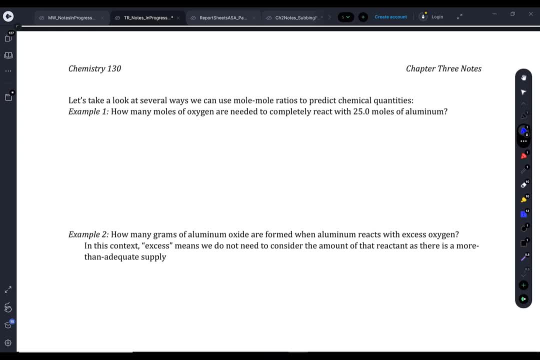 And I'm going to assign a lot of these for you to do on your own. Okay, So, using that equation, Okay, Okay. So using that equation, and I'm going to rewrite it again here, four moles of aluminum plus three moles of oxygen gives you two moles of aluminum oxide. 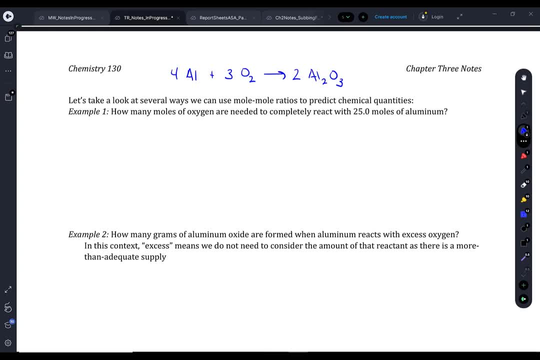 Let's go ahead and look at example one. How many moles of oxygen are needed to react with 25 moles of aluminum? This is unusually easy, but it's a good starting point. If I have 25 moles of aluminum, what ratio? 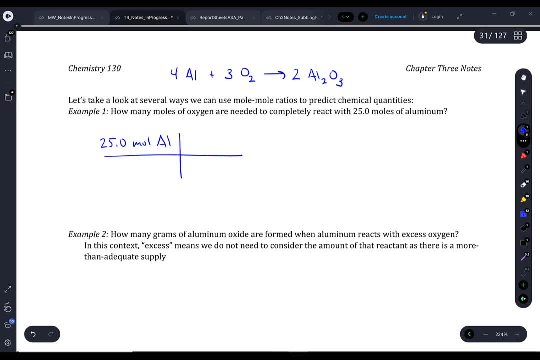 What ratio do I want? For every four moles of aluminum, I will need three moles of oxygen. Good, Okay. So that's 25 times three-fourths 4.75, is 18.8.. Okay. 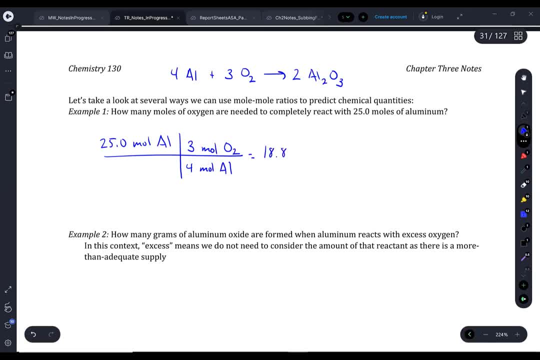 So that's 18.75, so that's significant digits. Wire meter round. Now in the real world. that's by itself not a very practical problem, because we're almost we don't have a mole meter in lab, right. 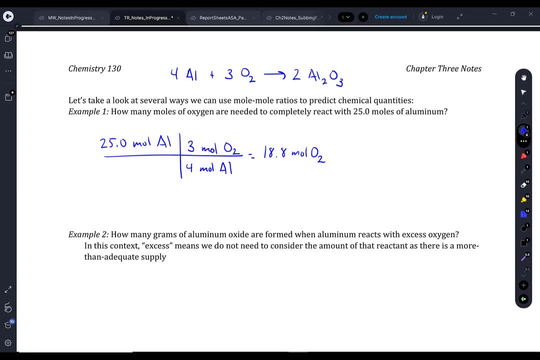 We have a balance. So you'd have to convert first from grams to Moles, right, Good, And I usually don't want to know the amount of the product. Well, gases, yeah, I might want to know those in moles, but I often want to know them in grams. 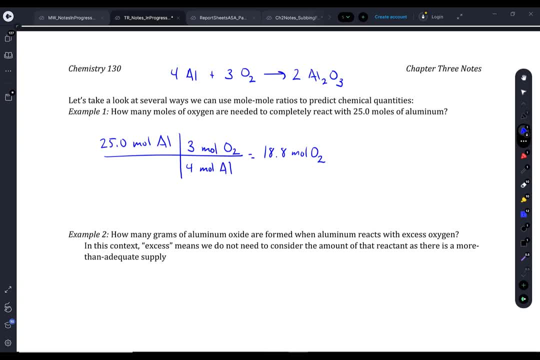 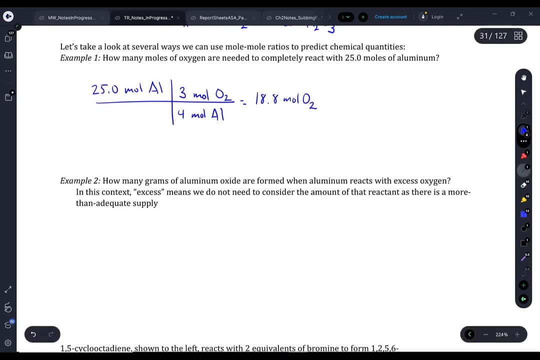 So same thing, I'd need to use the gram conversions. So example two is typical of probably the single most common calculation in all of chemistry, and that is going from the grams of a starting material to the grams of a product, or vice versa. 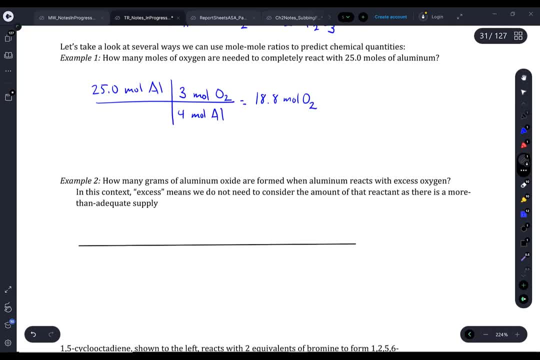 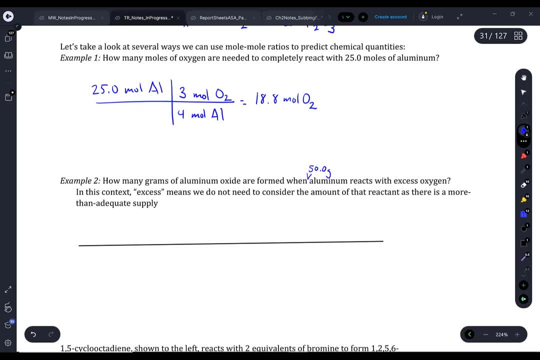 Let's say 50 grams. How many grams of aluminum oxide are formed when 50 grams of aluminum reacts with excess oxygen? So that word excess is so important. It means that there is more. It means that there is more than enough, so you don't need to consider it. 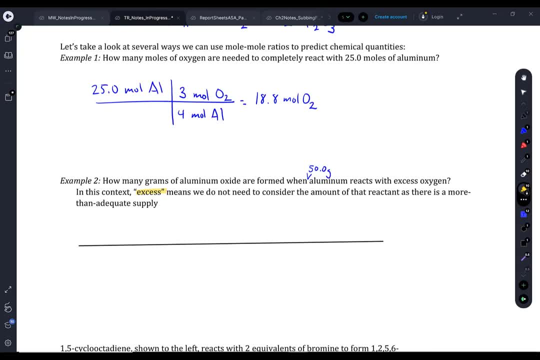 If I did give you an amount of oxygen, the problem becomes a little more complicated. It then turns into what is called a limiting reactant problem, which we'll talk about next. Okay, So the word excess means ignore the oxygen, only consider the aluminum. 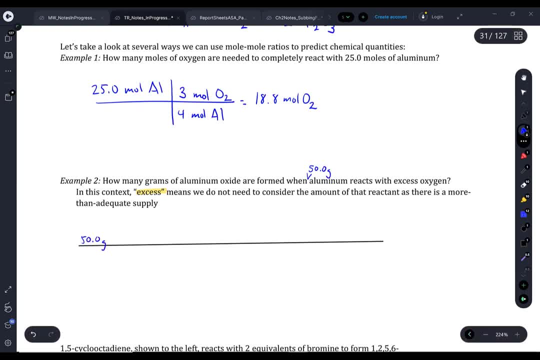 So if I have 50 grams of aluminum, I'm going to have to consider the aluminum. So if I have 50 grams of aluminum, we're just going to do very similar to what we did in the last problem. We first need to get it, though, into moles. 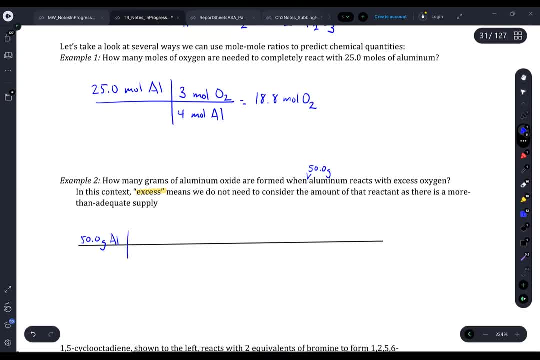 Yes, So what number do I need? here We're going from grams of aluminum to moles. Good Yeah, the atomic weight of aluminum is 26.98.. Good, So I've got 26.98 grams of aluminum is. 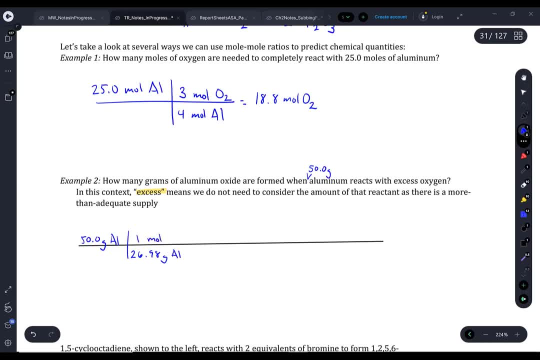 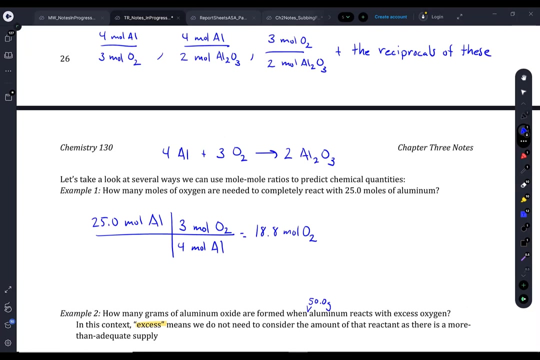 A mole of aluminum. We're trying to figure out what, How much aluminum oxide. So we're going to need the mole-to-mole ratio of aluminum and aluminum oxide. And we see up here it says: four moles of aluminum make two moles of aluminum oxide. 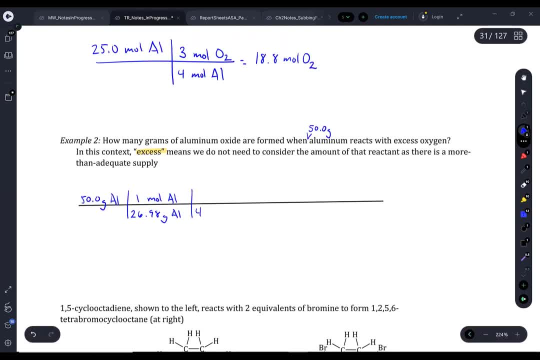 Okay, All right, So let's do what It's light. It's light. It's too big. All right, So let's go ahead and convert moles of aluminum oxide to grams. I think it's 100 and something. 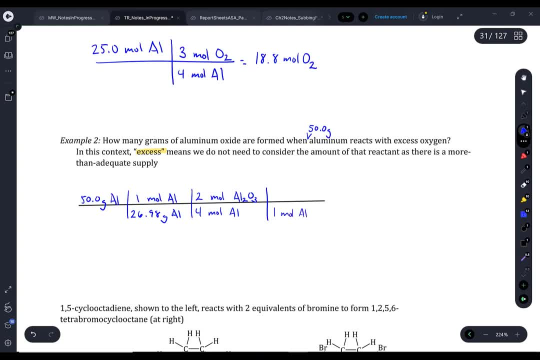 So one mole of aluminum oxide. So aluminum is 26.98, 2 times 26.98, right Yeah, Plus three oxygens, that would be 48.. So I'm getting 101.96.. You notice, everything cancels nicely in terms of my units. 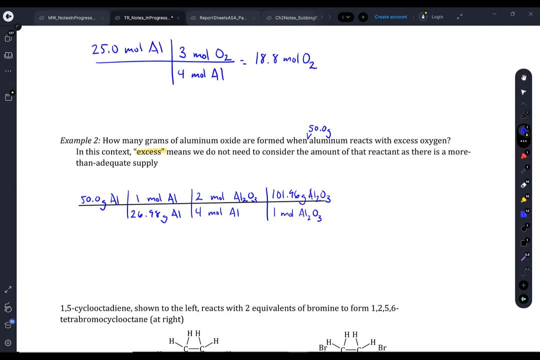 to leave me only with grams of aluminum oxide. Please learn to do the problems this way. okay, Because I'm generally not very generous on partial credit if I can't very quickly figure out what you did. If you want to do the problems this way, 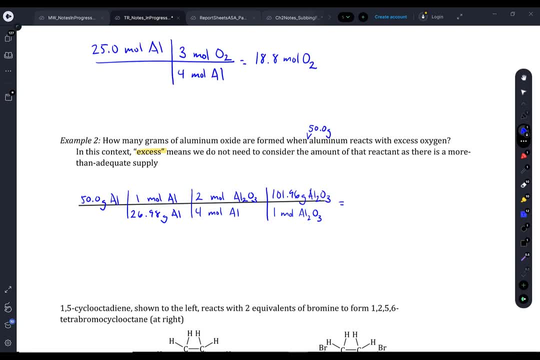 you've got numbers all over the place, I'm just going to go- yeah, no, I don't get it- and not partial credit. So what you need to do needs to do it, you know, be written nicely as close to the style that we're doing it this way. 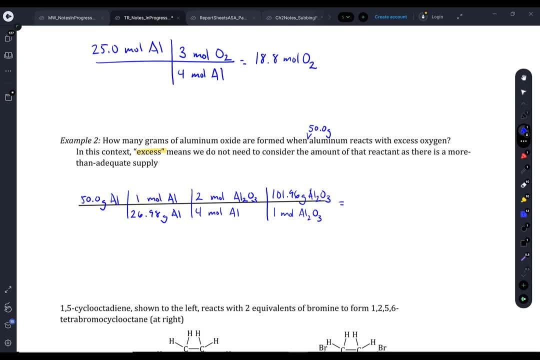 And this is how your textbook does it. It's how every textbook does it, So chemists understand it. Make sure you write it out in this style: I'm getting 94.8.. Five, don't you got it? Any questions on that? 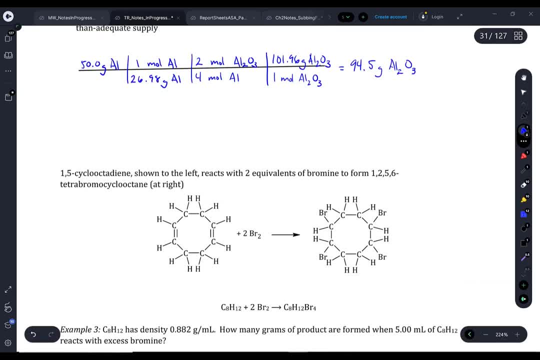 No, All right. so the next section here says: I've got 1.5-cyclo-octadiene, which is this chemical right here. reacts with two equivalents of bromine and makes 1,, 2,, 5, 6 tetrabromocyclo-octane. 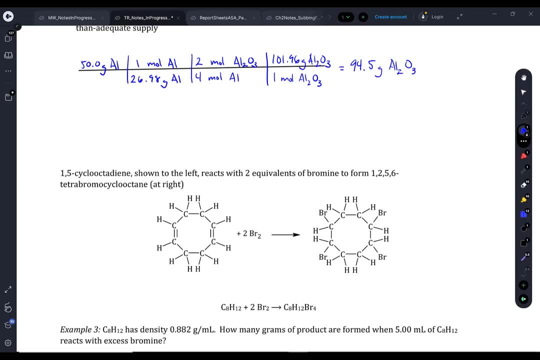 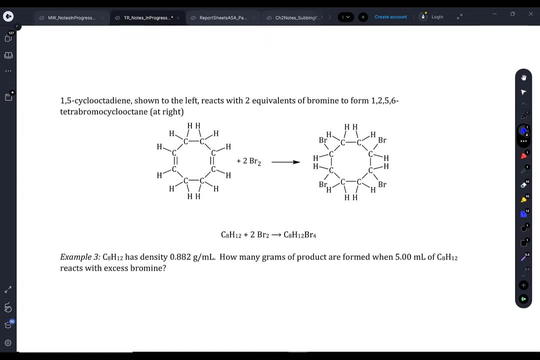 Don't you love this? You haven't. that's what organic naming starts looking like, So it gets much more involved. Now, that's all ugly, so we don't need this level of detail In these kinds of problems. so instead of using these structural formulas, 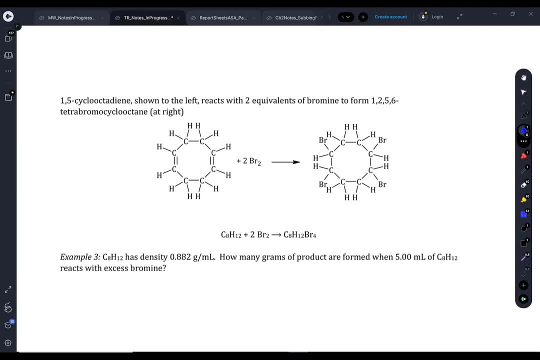 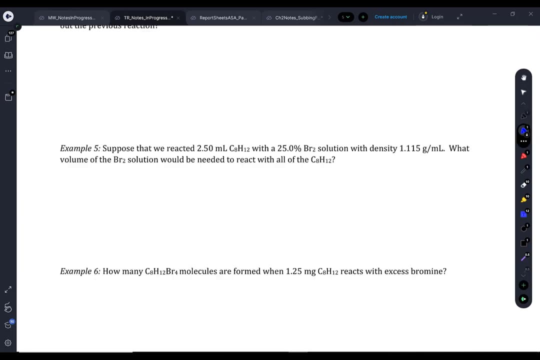 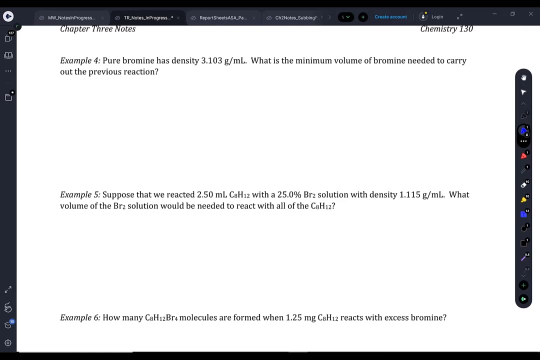 or Lewis structures. let's just rewrite everything as these guys right here. Okay, So I'm going to do example three, but I will leave the rest for you to do. Wait, we're done at 350, right? Yeah, I think I can do this question. 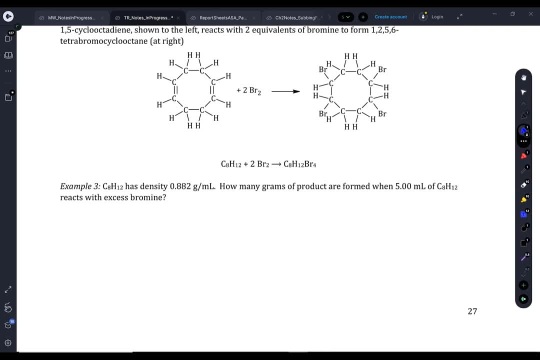 I have time to do this question, All right, so let's start off first of all by finding the molecular weight of everything, Because it'll just be easier. So, if we have C8H12,, C8H12 is 12.01 times 8.. 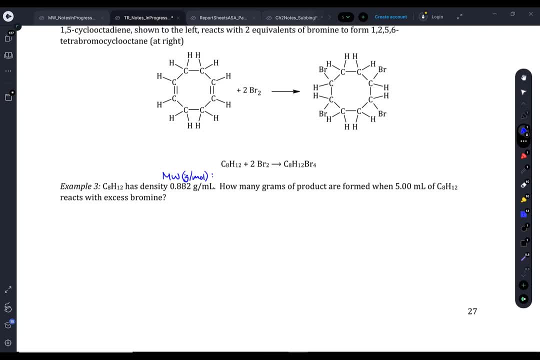 Plus 16 times 1.00,- I'm sorry, not 16,- 12, times 1.008, I'm getting 108.18,. yes, It may not be apparent, but it would be easier now to go to the last thing. 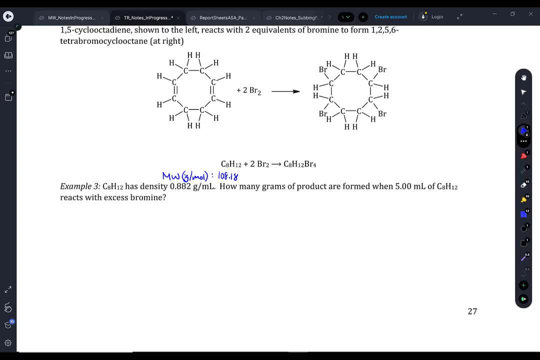 So I'm just going to take a look at this, Okay, Because it's C8H12, right, So I'm going to take that plus add the four bromines, which are 79.9.. So these are 427.78.. 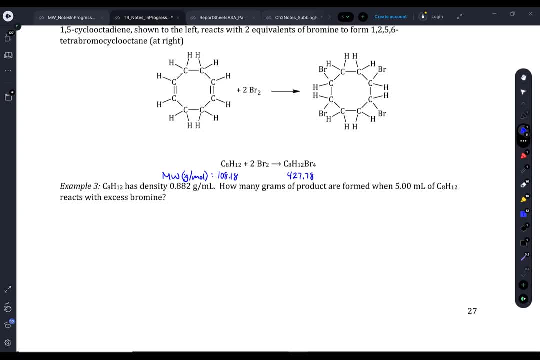 And then bromine. I don't count the two in the front right. Molecular weights are just the. It's just the formulas. So molecular weight of bromine is 79.9 times 2, 159.8.. But you agree, if I took this number- 108.18, plus two times this number, it should give you the same number as this right. 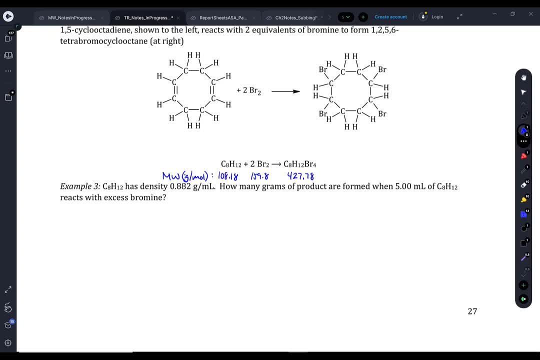 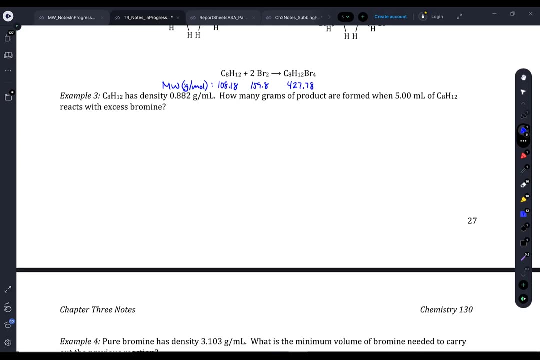 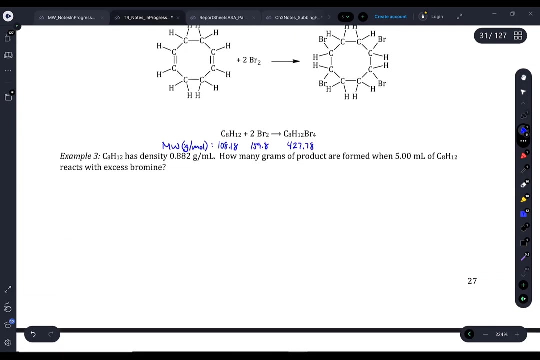 Okay, Because you see all the atoms get accounted for Good, Okay. So that said, so we will say that our starting material here- so we'll say spider with double bonds, has this density: How many grams? How many grams of product are formed, if I start with five milliliters of that? and it reacts with excess bromine. 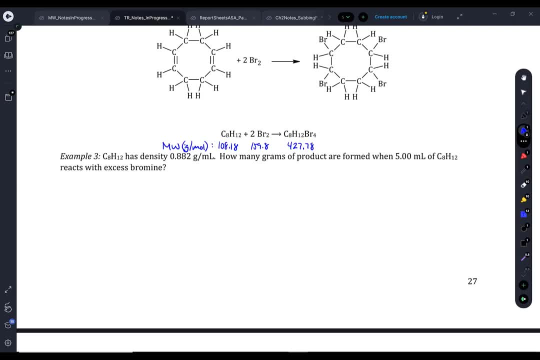 Excess again means I can ignore the bromine. There's more than enough of it. This problem is very, very similar to the last problem. The only difference is, instead of starting with grams, I'm starting with- yeah, milliliters. 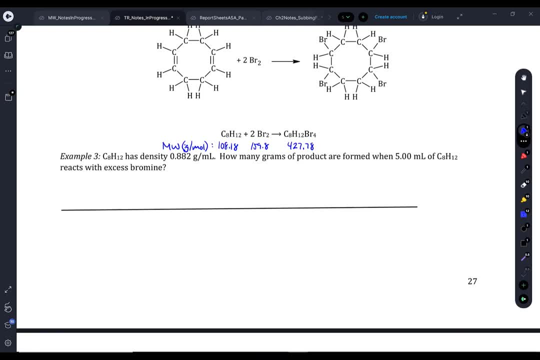 Why wouldn't I start with the density, by the way? Okay, Well, what's been my advice to you against that? Yeah, don't start with ratios, units that are ratios. The point of those ratios is to act as a conversion factor. 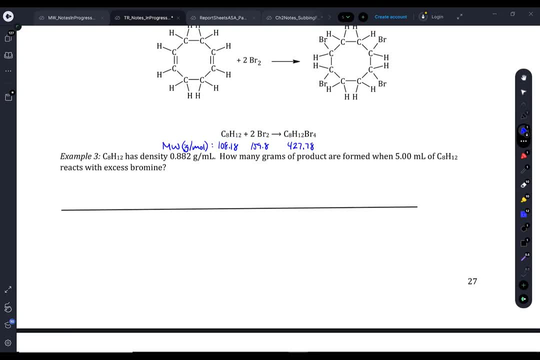 Yeah, Good. So I'm going to start with the five milliliters of crazy double bonded spider C8H12.. And I need to get to moles, but I can't go milliliters to moles, but I can go milliliters to grams. 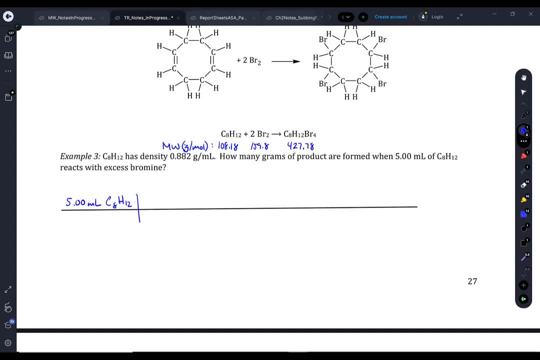 Good. So where am I going to do that? I'm going to say, well, there's 0.882 grams of it for every one milliliter, right? So every one milliliter of this compound has 0.882 grams. 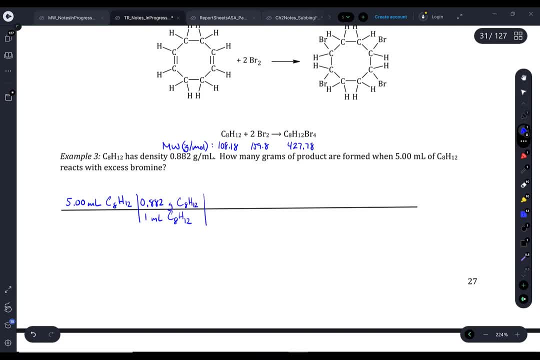 And now I need to get that from grams to moles. So that's why I calculated the molar masses first. There are 108.18 grams of this in a mole. Okay, And we're trying to get to grams, Okay. 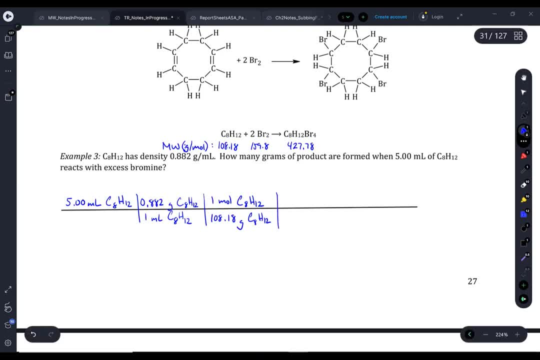 And we're trying to get to grams of the final product. So what do I do here? I say, well, mole to mole ratio is every mole of the starting material. I should have done this the lazy organic chemistry way, which is to call this one and call this two. 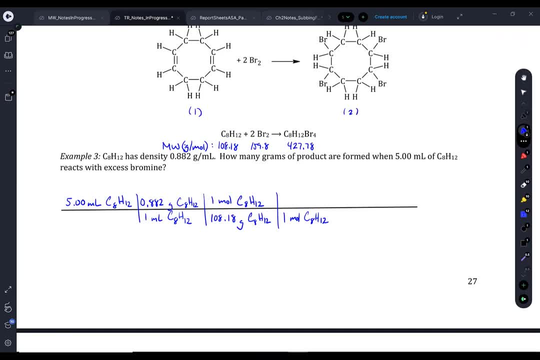 So we're going moles of one to moles of or A, B, right, That would probably be the easier way to do it, but anyway. So, in any case, one mole of that gives you one mole of the final product, C8H12Br4.. 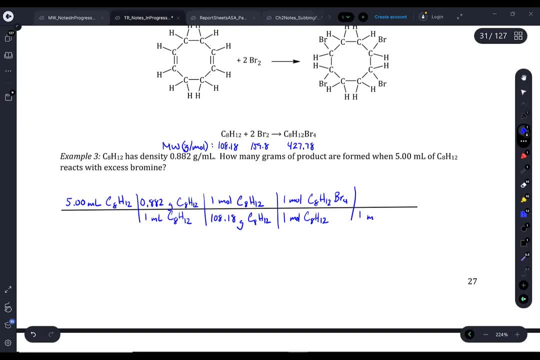 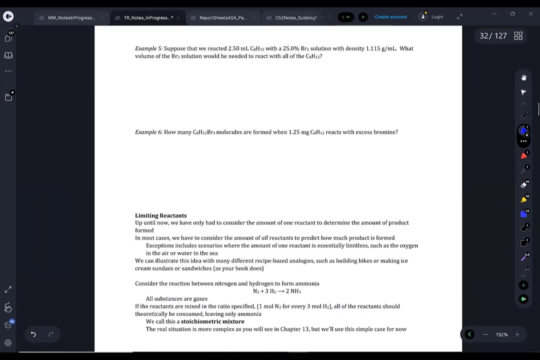 And we've already calculated its molar mass. one mole of that- And because I'm running out of space, I'll just say is 427.78 grams, And I'm going to leave that to you to calculate. okay, And I would like you to also do. 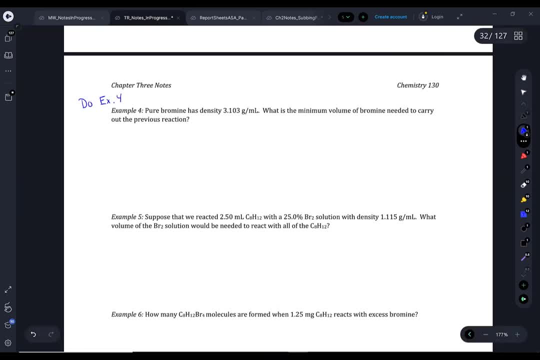 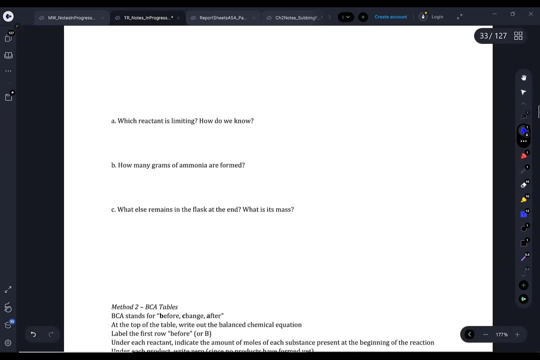 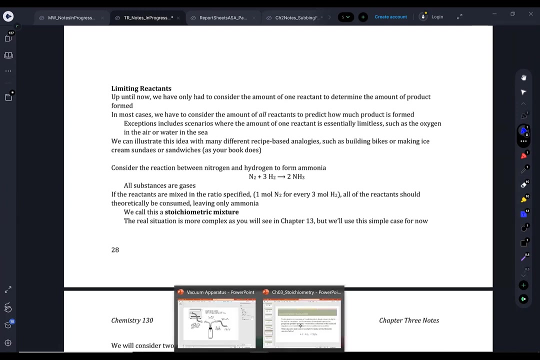 Okay, Example four to six for Thursday, so that I can get ahead right now. Sorry, I rarely let people out early, Because I want to at least talk about limiting reactants, A vitally important subject that I saved for last here. 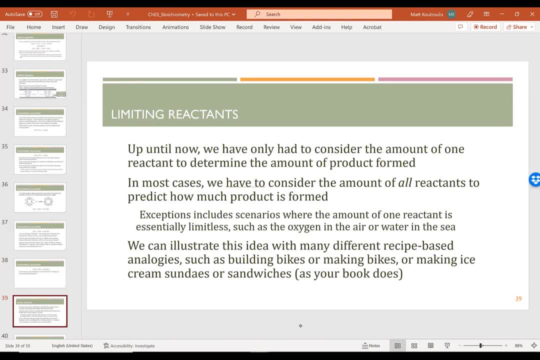 But one of which you should be familiar. Okay, so for right now, I've only asked you to consider one reactant at a time, And if we had another reactant, I've said it was what In excess, which means we don't have to worry about it. 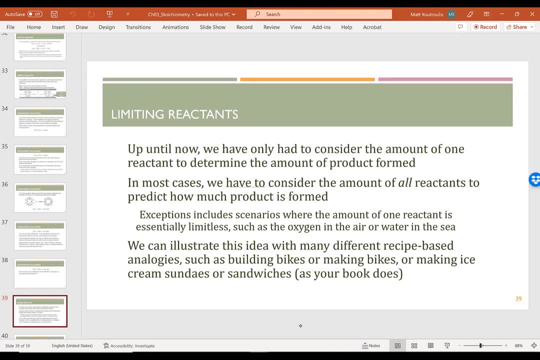 What that means is the chemical I specified is what's called the limiting reactant. In theory, this is the chemical you will run out of. okay, Once you run out of it, the reaction cannot go forward. That's what a limiting reactant is. 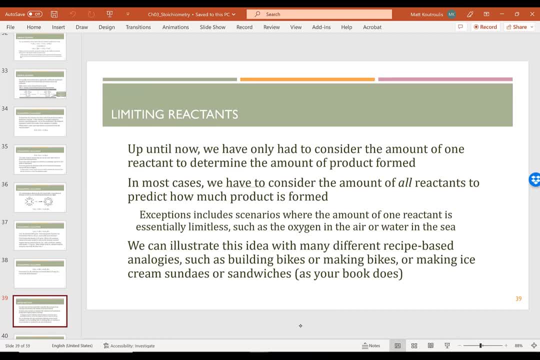 Now, in most reactions I'm telling you not how much of one reactant there is, But you would want to know the amount of all reactants And only one of these would generally tell you essentially how much there is of a certain substance. 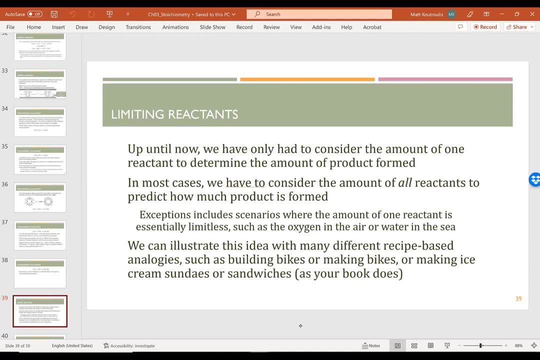 Certain things are almost always limiting or are almost always in excess, Like, for example, oxygen gas. Why is oxygen gas virtually always in excess? If it's done in the open air, it's in excess Because it's in the open air. Because, yeah, it's limitless. If oxygen gets pulled into your reaction, there's still going to be more. The only time it's not limitless is if you do it in a sealed container, Because then eventually the oxygen could run out if no new oxygen can come in to fill the place of the others. 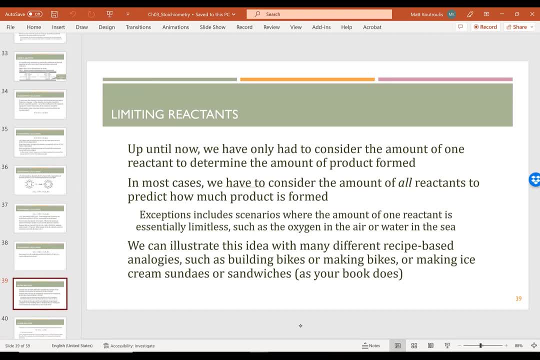 There are many, many different ways that we can illustrate the concept of limiting reactants. We can use bicycles, which is, I think, what the textbook does. We can use ice cream sundaes- I do in Chem 120, where I say: well, you need two scoops of ice cream plus one cherry, plus 50 milliliters of chocolate syrup. 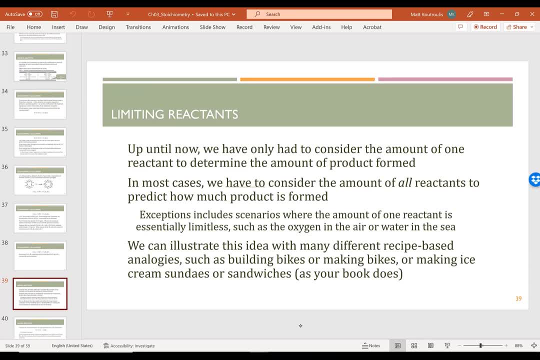 Because we always measure chocolate syrup in milliliters, And that is one sundae Right? It doesn't matter if you have 1,000 cherries, If you only have four scoops of ice cream, you're only going to get two sundaes. 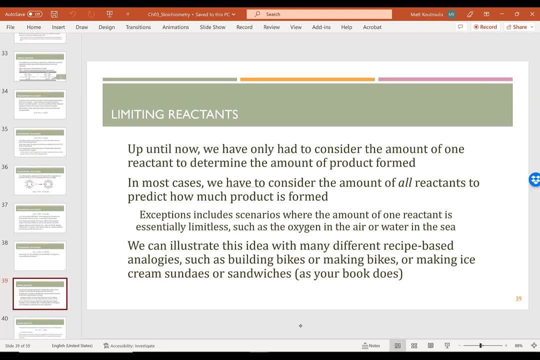 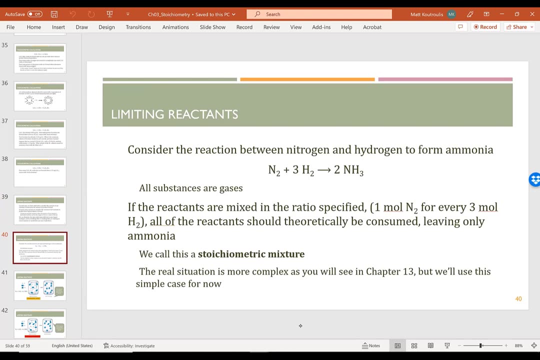 Does that make sense? Good, The cherries are excess, And sandwiches? that's another case. That's what the book does, is sandwiches OK. So we're going to look at a very common reaction that comes up a lot in this class. 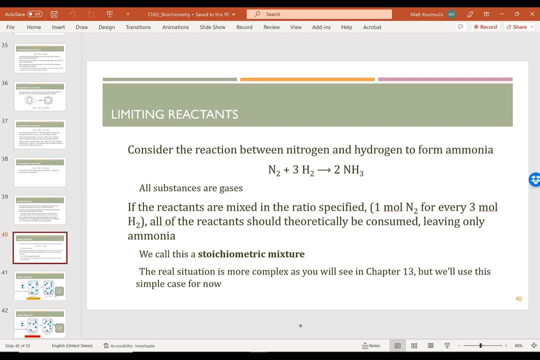 So I am showing the reaction of nitrogen with hydrogen to form ammonia. This is called the Haber process. Anyway, it even gets a name. It's so famous. Everything I tell you about this reaction this semester is a complete and total lie. 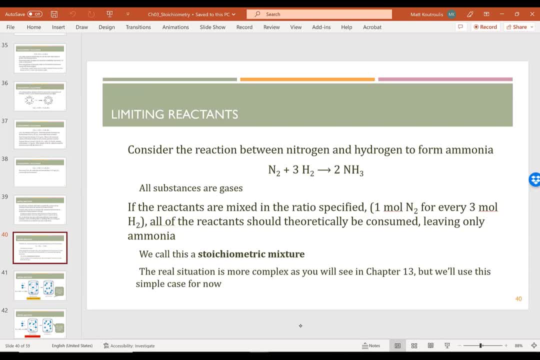 OK, OK, We're going to say that one mole of nitrogen plus three moles of hydrogen gives you two moles of ammonia. That never happens Because we are totally ignoring a critical problem that we will deal with in Chapter 13, called equilibrium. 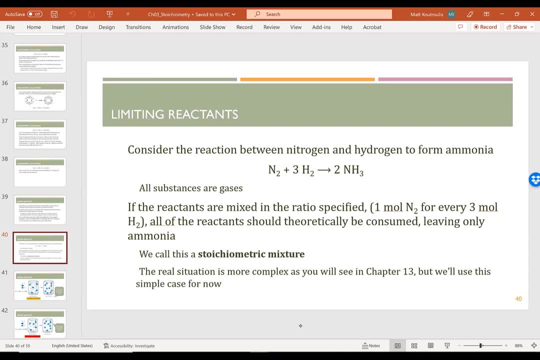 This reaction only goes partway and then it gets stuck, And that's true of most reactions. They get stuck. They come to what's called an equilibrium. We are going to go through the lie of saying it doesn't get stuck, OK. 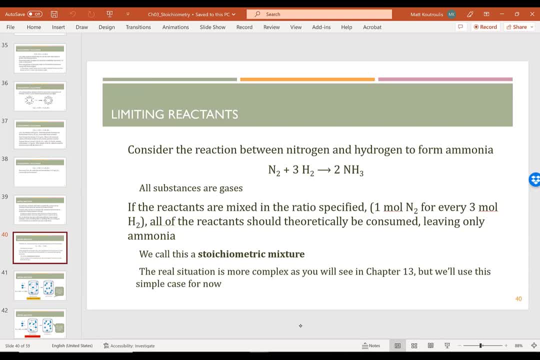 And it will go all the way to the end. So just you know, sometimes that might happen and it might take five million years, But I don't care if it takes five million years, It does eventually happen. So what we're going to say here is what if you do this as follows: 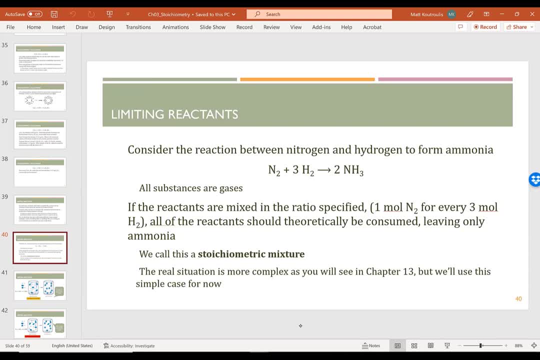 What if I do take one mole of nitrogen and three moles of hydrogen, Assuming the reaction goes to completion? this is what's called a stoichiometric mixture. That means they're technically Isn't a limiting reactant, because you're using exactly the right ratio: one mole, two, three. 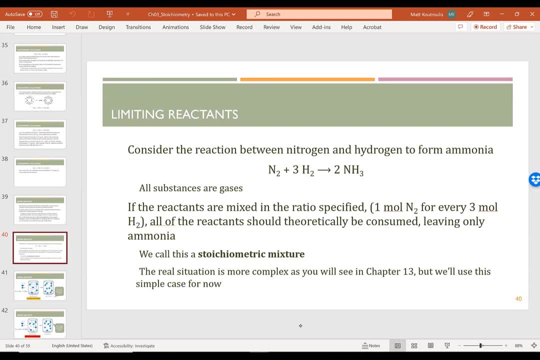 And if the reaction goes to completion, you would get two moles of ammonia. What if I used 10 moles of nitrogen and 30 moles of hydrogen? That's stoichiometric, because I've multiplied both of these by 10, and I should get 20, right? 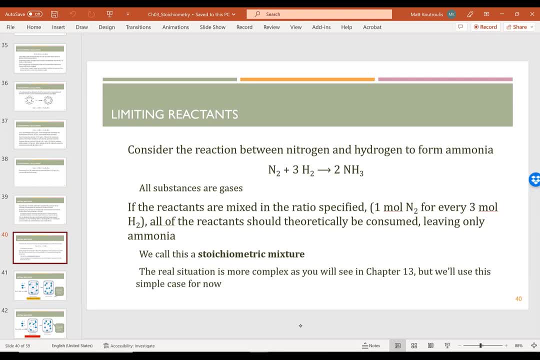 What if I used 50 moles of nitrogen and three moles of hydrogen? That's not stoichiometric. That means I'd have a lot of nitrogen. That's not stoichiometric. That means I'd have a lot of nitrogen. 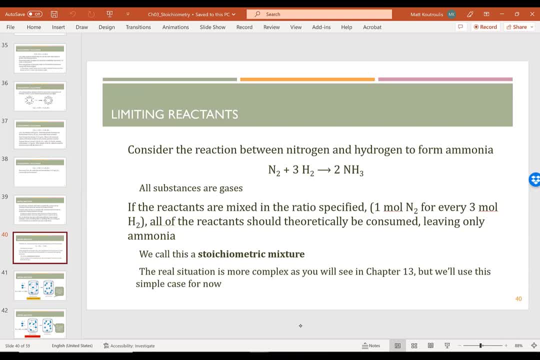 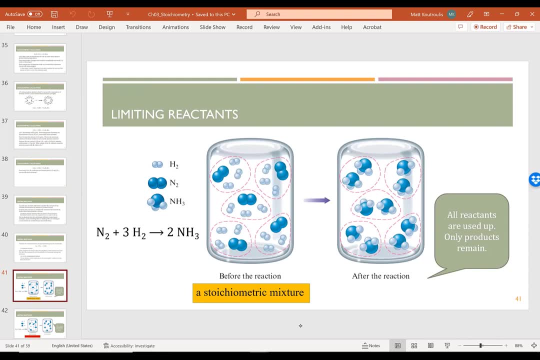 That means I'd have a lot of nitrogen left over. Nitrogen is in excess. So let's take a look at a stoichiometric mixture from the textbook. What we're doing here is so here are all our reactants This picture is showing. what we've done is we've taken all of these and we've circled them so that in every circle there is a nitrogen molecule and three hydrogen molecules. 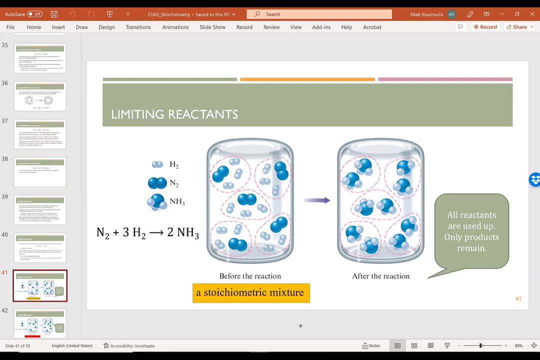 And there is nothing. And there is nothing left out of any of the circles right And there is nothing left out of any of the circles right. So this is illustrating a stoichiometric mixture. What this means is: at the end, all the hydrogen and all the nitrogen have been converted into ammonia. 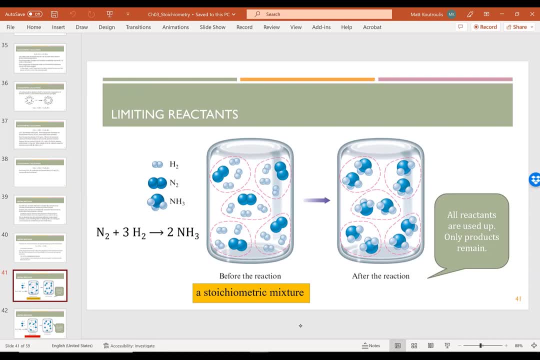 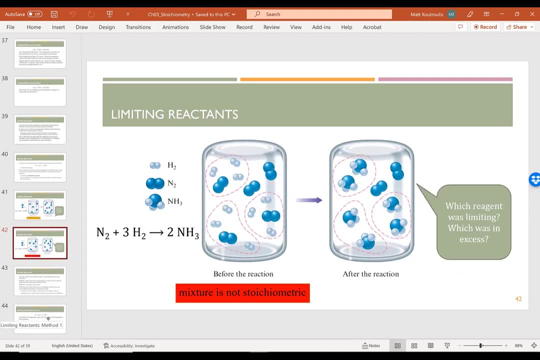 What this means is: at the end, all the hydrogen and all the nitrogen have been converted into ammonia, Agreed, So every circle now has two ammonias, And so these are very rare that we do this. This is much more common, So this is not stoichiometric. 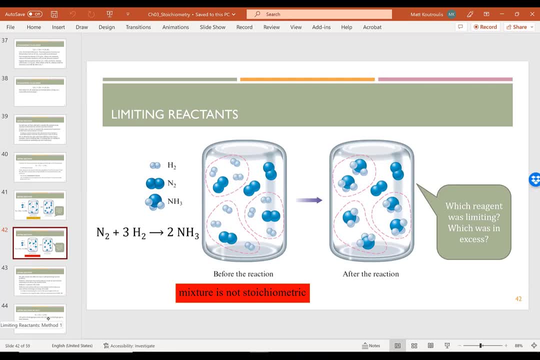 What this is saying is OK. we added this, but I wasn't able to find a place for these nitrogens. So we say the nitrogens are in excess. Good, And you'll notice that when we go to the circles, each of these circles now has two ammonias, but there's still nitrogen left. 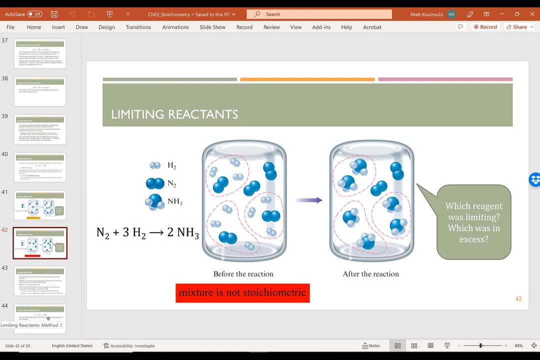 So if I ask you, you know what's the total amount of product. You can't just say it's the ammonia, There's still nitrogen. Does the mass of the product change? Does the mass of each still remain the same? The total mass? 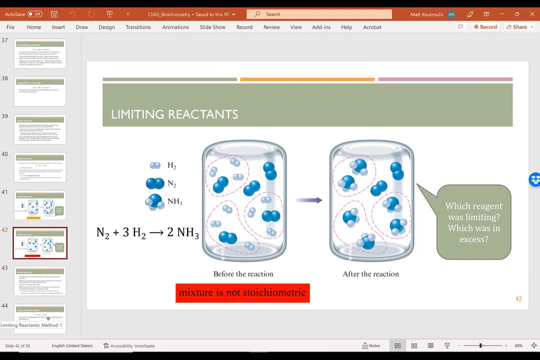 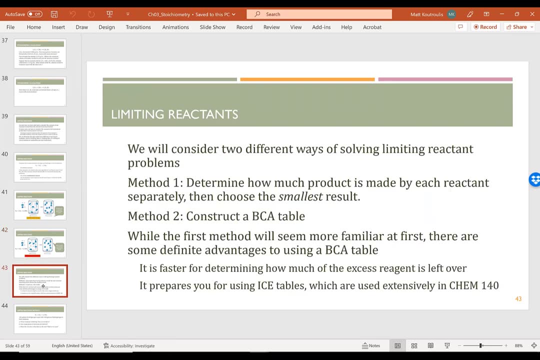 Yeah Good, But you can't say it's just all ammonia. So we would say the M2 is in excess. OK, Now we're running out of time here and that's fine. I'm a little, actually, behind the other class, but we're going to look at two ways of solving these limiting reactant problems. 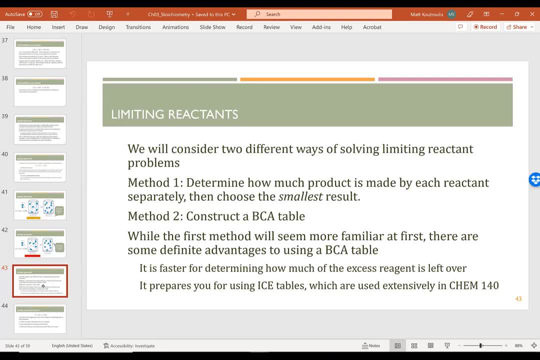 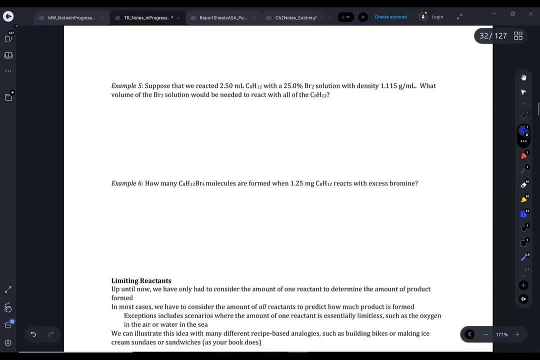 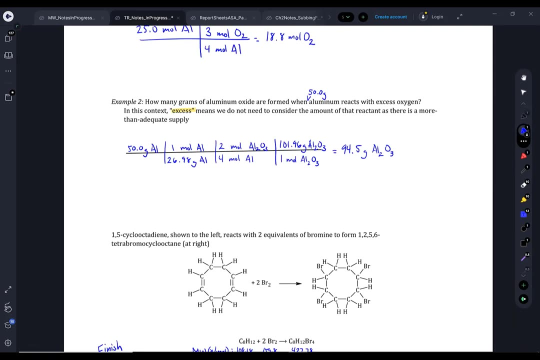 And I will start those on Thursday. We're going to do it the way that we learned in Chem 120., Which is you do this problem grams to grams for both reactants. So, for example, if I told you the grams of aluminum and the grams of oxygen, you would do the grams of aluminum and grams of oxygen in a separate problem. 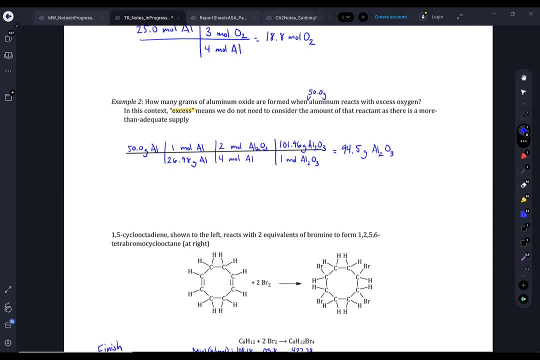 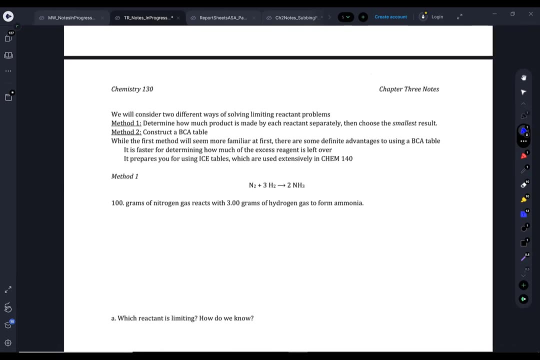 And which would be the correct answer. It's always the smallest answer, We all remember that- And the larger answer is M2.. The larger answer is junk. It's totally useless. Now. that method works well most of the time. The other method which most people hate initially is the BCA table method. 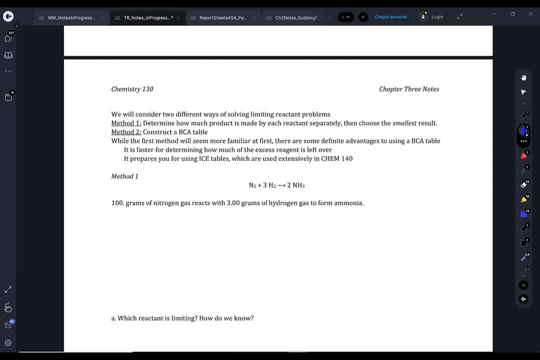 The second method is much better. when you need to know exactly how much of everything is left over at the end, Does that make sense? So when I need to account for everything- and in Chem 140 especially, that's critically important To know how much there was before and how much of everything there is at the end. 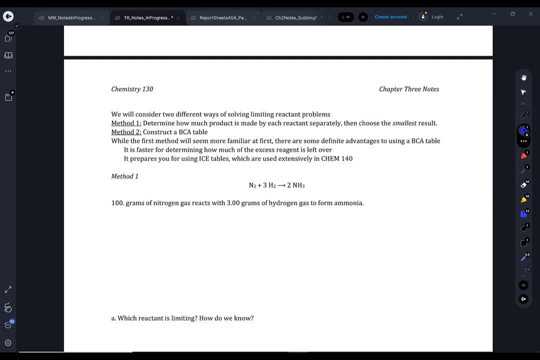 And so the BCA table method works much faster for that. It also works much faster when you're dealing with net ionic equations and milliliters and molarity. So I'm going to introduce it on Thursday but we're not going to make really extensive use of it until starting in Chapter 4..